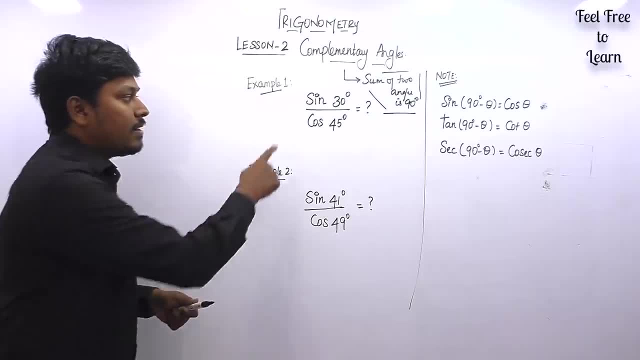 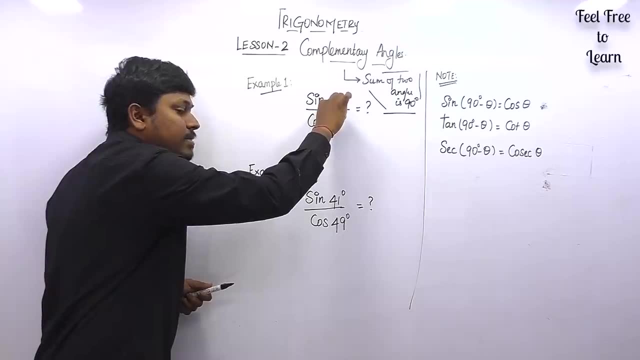 which example is a complementary angle and which example is not a complementary angle. See here first example: sin 30 degree cos 45 degree. Here they have given two angles. whether the sum of two angle is 90 degree? No, once you add two angle, 45 degree plus 30 degree, resultant will: 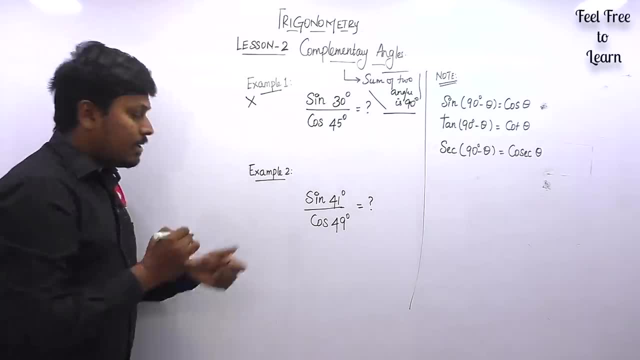 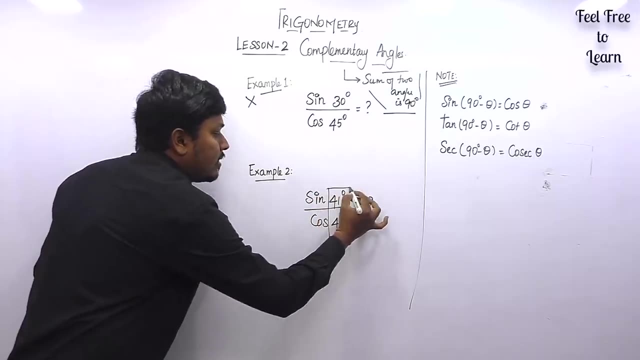 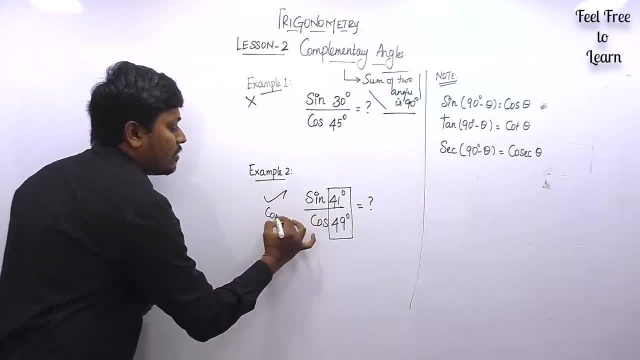 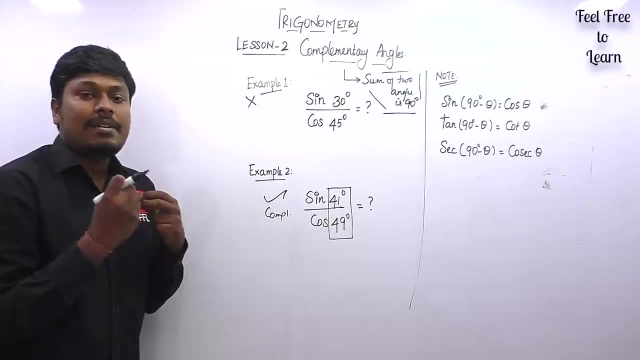 90 degree. So we can say we can solve this question by using a complementary angle concept. Got it, friends? that is it. So while solving a trigonometry question, first you guys have to check whether the question is complementary angle or a normal trigonometrical ratios. You can see: 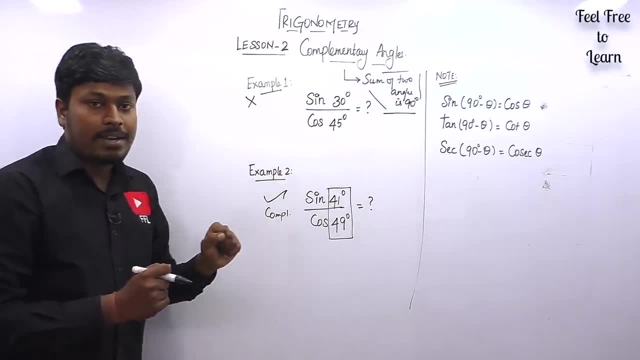 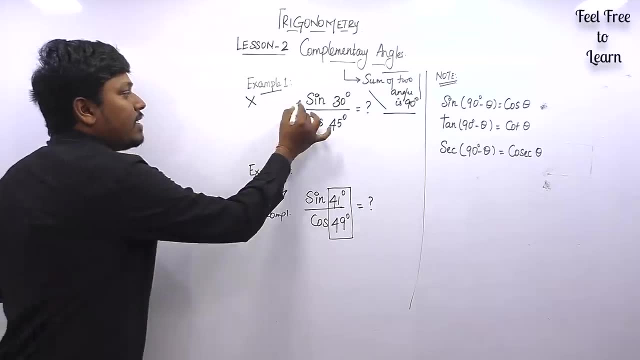 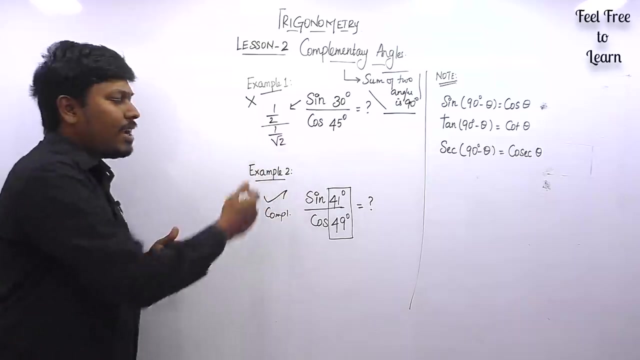 example number 1, sine 30 degree divided by cos 45 degree. In lesson number 1, I have clearly explained what is called as direct trigonometrical ratios. What is sine 30 degree? Sine 30 degree will be 1 divided by 2.. What is cos 45 degree? Cos 45 degree will be 1 divided by root 2 and you. 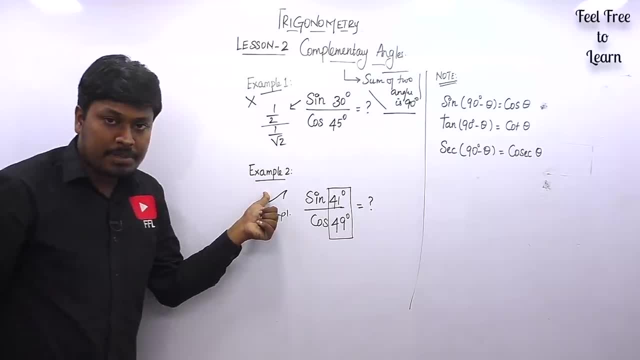 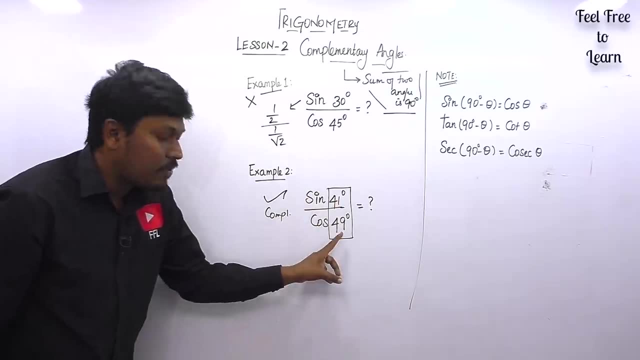 can solve this question completely. But when you look at the example number 2, where sine 41 degree, it is not a direct trigonometry ratio. So for the sine 41 degree and cos 49 degree we found that it is a complementary angle. So if it is a complementary angle you need to buy out the 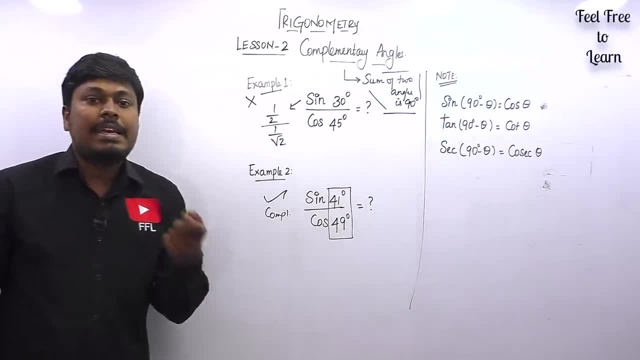 simple logic. That is what is sine 90 minus theta. Sine 90 minus theta will be cos theta. Tan 90 minus theta will be cot theta. Similarly, secant 90 minus theta will be cos theta. You do not want to buy out this right. It is simple. Listen here. sine is equal to cos tan is equal. 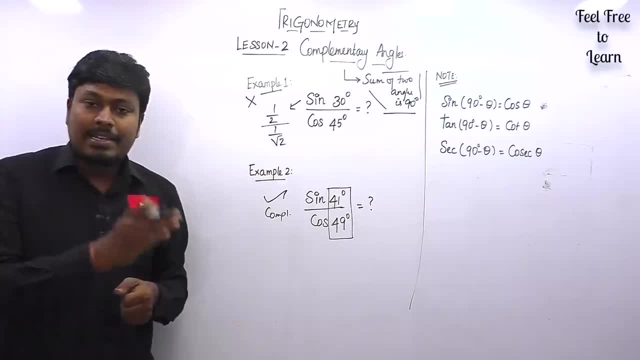 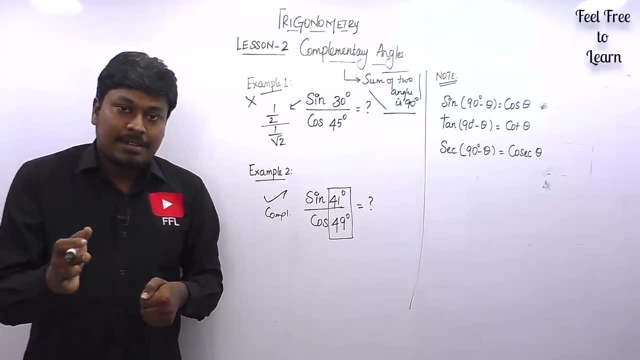 to cot secant is equal to cos theta. That is it. Friends got it. Sine 90 minus theta is equal to cos theta. Cos 90 minus theta is equal to sine theta. Tan 90 minus theta is equal to cot theta. 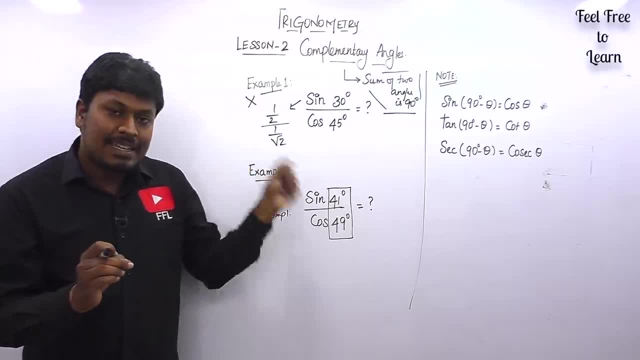 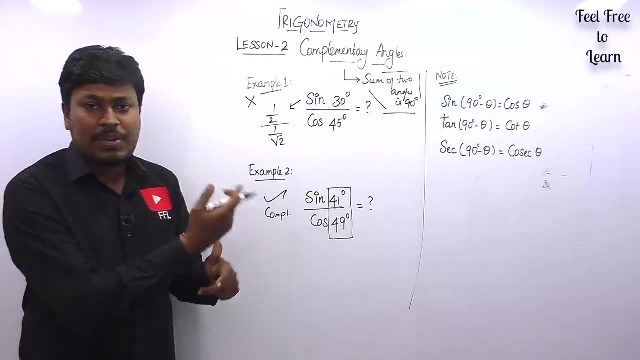 Cot, 90 minus theta is equal to tan theta. Then last, secant, 90 minus theta is equal to cosecant theta. Cosecant 90 minus theta is equal to secant theta. And if theta is an acute angle, you do not want to remember all those stuff. It is enough to buy out only these three formulas. 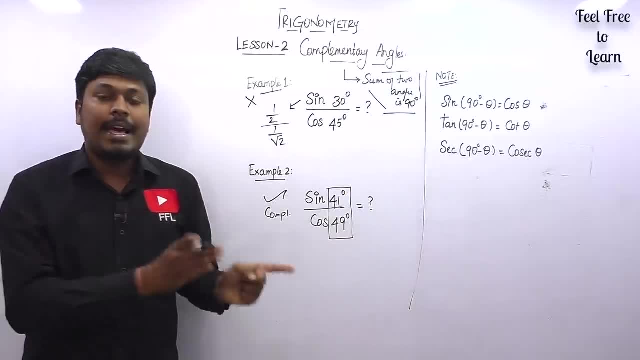 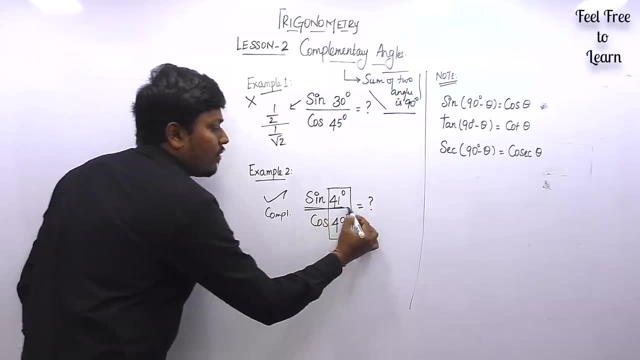 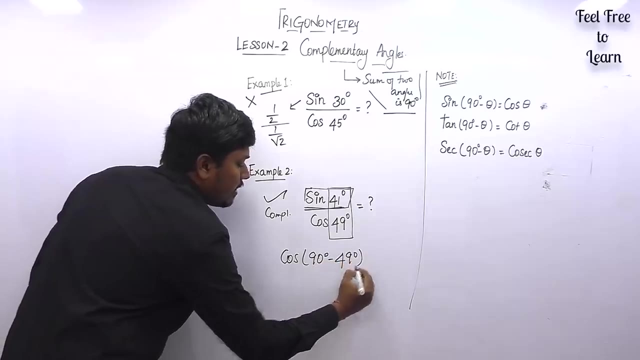 Got it, friends. So simple logic: sine is equal to cot tan equal to cot, secant is equal to cosecant. So we will be applying the concept here. Just I can solve this question. See here: sine 41 degree. how I am going to write this: as cos of 90 degree minus 49 degree divided by 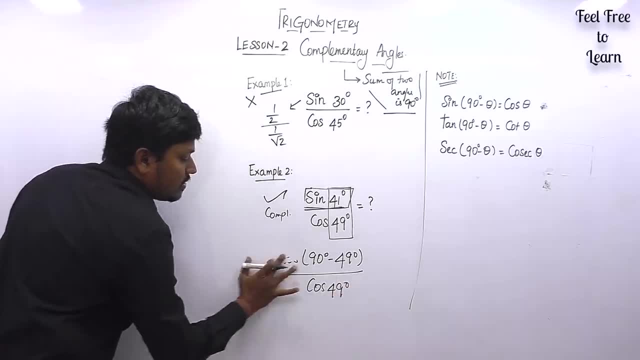 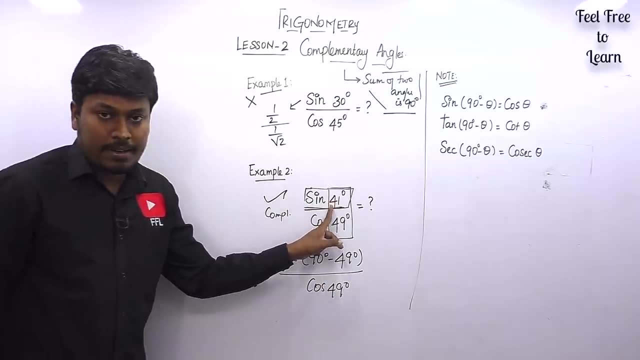 cos 49 degree. Friends got it. Sorry, sorry sign, This is sine, Friends got it. What I have done is here we found the numerator sine 41 degree. So sine 41 degree can be written as: 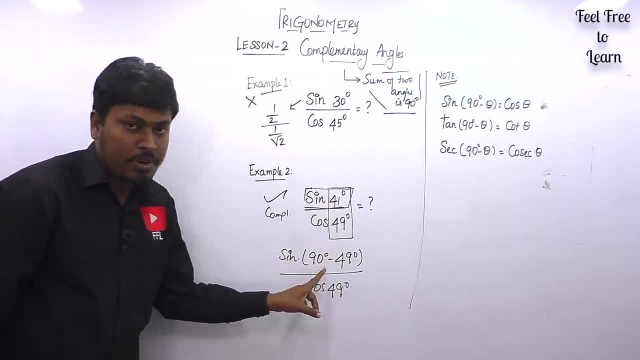 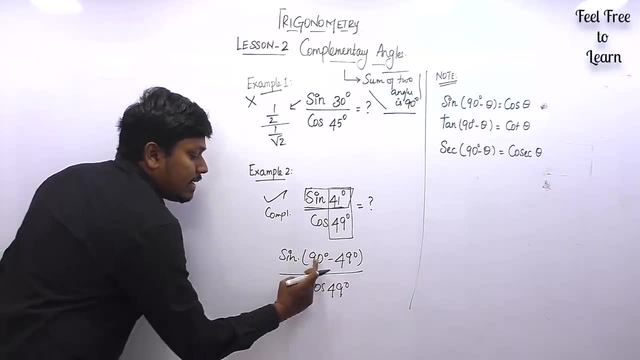 90 minus 49.. What is 90 minus 49 will be 41.. So finally, I am writing the numerator as sine: 90 degree minus 49 degree. So 90 minus theta. sine 90 minus theta will be cos theta. So we can. 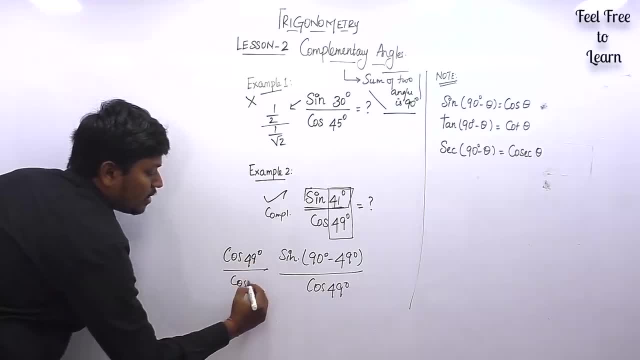 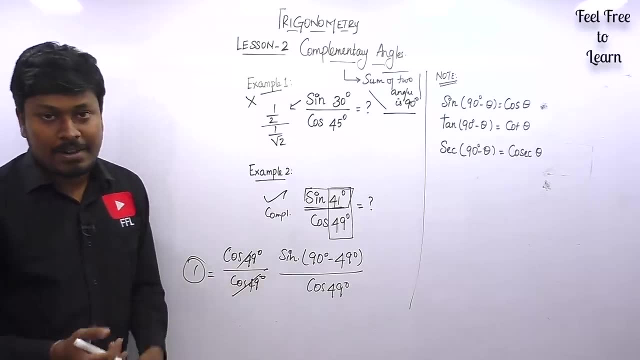 say this as cos 49 degree. Similarly, denominator cos 49 degree. we can cancel both the terms and we can say the result and answer will be 1.. Friends got it. It is called as a complementary algorithm, Simple concept. you can either convert: 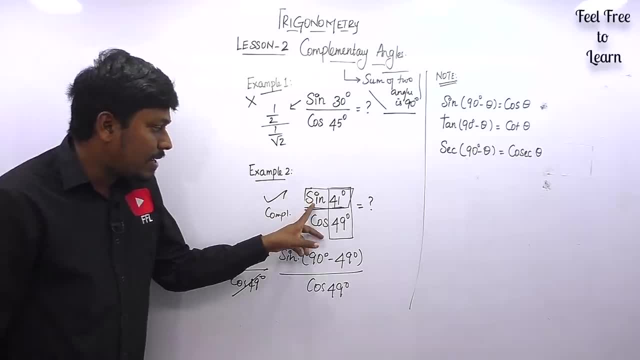 the denominator or otherwise numerator, If you want. you can write this as sine 90 minus 49, or otherwise you can write the denominator as cos 90 minus 41 degree. Either way you can going to get the same answer as 1.. So friends got it. So, before solving this 10 to 15 question, you guys 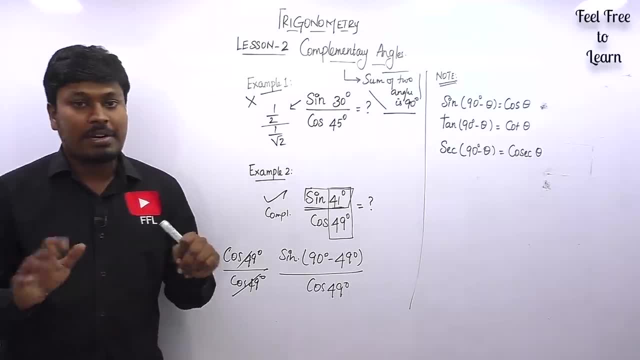 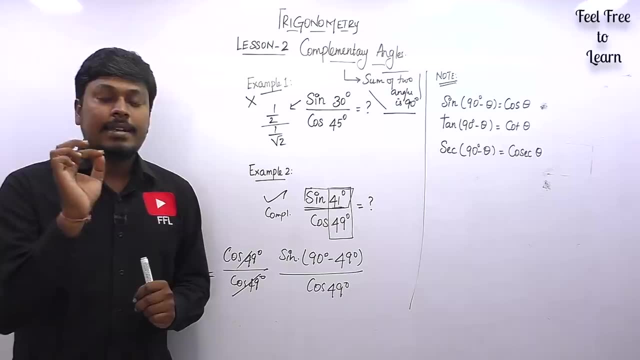 have to know what is called as complementary angle. Complete trigonometry topic. What is called as complementary angle? So the angle is said to be complementary. If sum of both the angles are 90 degree, 9, 0 degree, then it is called as a. 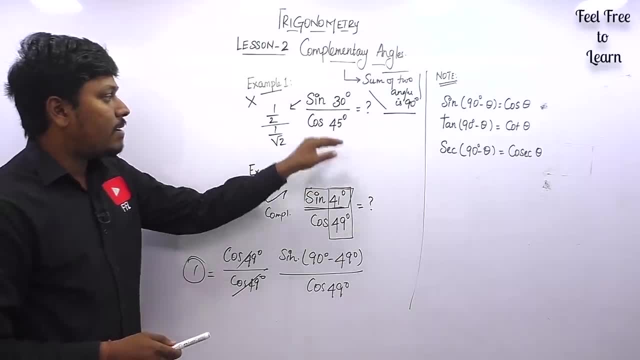 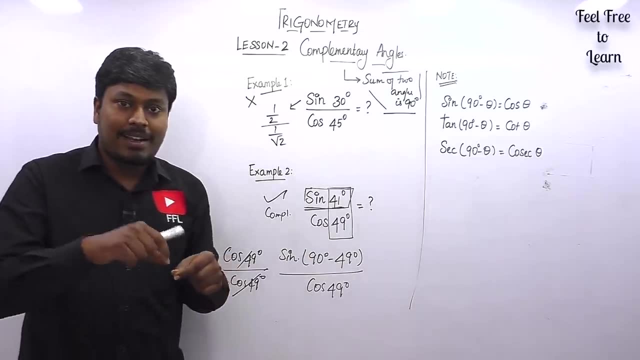 complementary angle Got it. So this is the difference between complementary angle and a non-complementary angle. So again, you do not want to buy at this. We are not kids to buy at write and writing every time in a paper and buy atting this. Remember that sine is equal to cos. 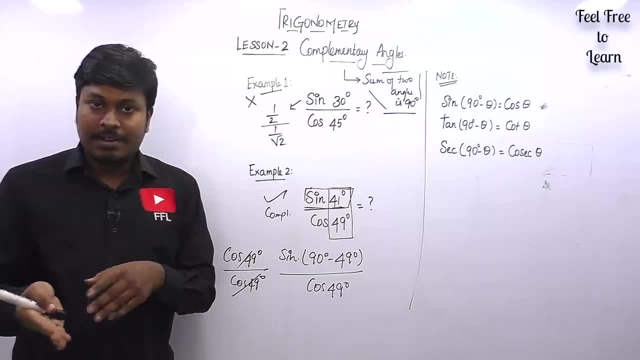 Again I am saying: sine is equal to cos, cot is equal to tan, secant is equal to got it. Sine 90 minus theta will be cos theta. Cos 90 minus theta will be sine theta, Tan 90 minus. 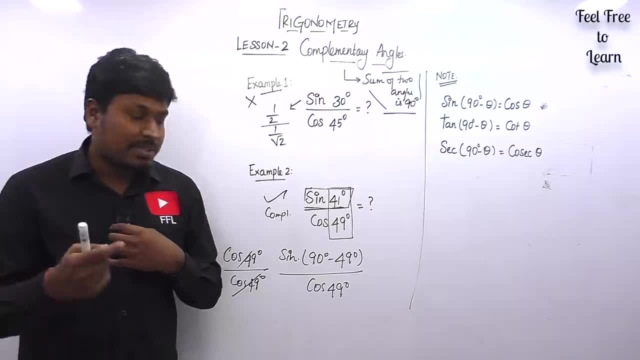 theta will be cot theta. Cot 90 minus theta will be tan theta. Cosecant 90 minus theta will be secant theta. Secant 90 minus theta will be cosecant theta. Got it. So let me move on to all the 15. 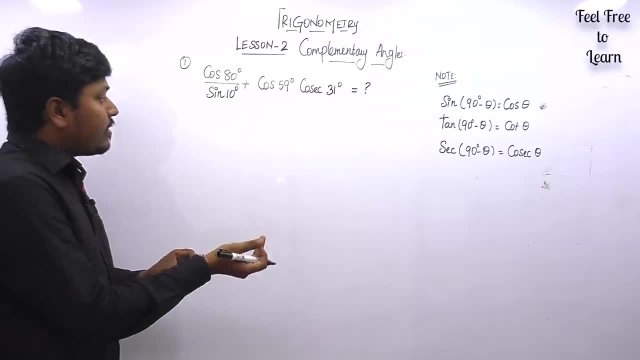 questions. Question number 1.. So cos 80 degree divided by sine 10 degree, plus cos 59 degree, into cosecant 31 degree, equal to question mark. So by seeing this question first, what you guys have to do is you have to find out what is a complementary angle or a direct trigonometrical value. 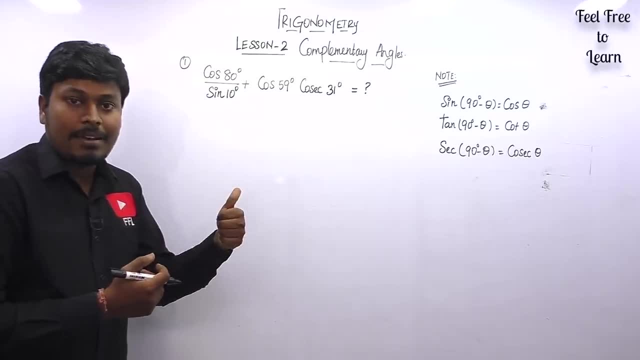 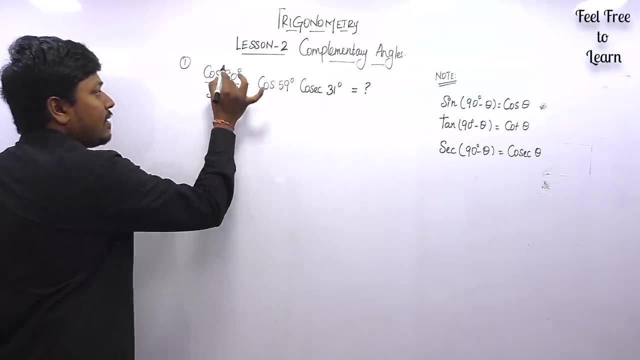 trigonometrical ratios, Whether it is a direct trigonometry or complementary angle. it is a complementary angle Why? Because listen here- first angle is 80 degree and the second angle is 10 degree, So we can say sum of angles are 90 degree, So we can say it is a complementary. 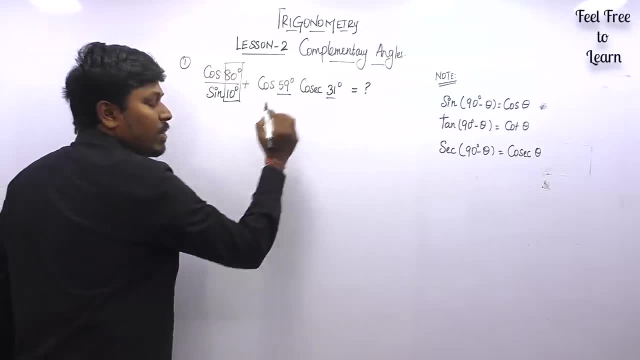 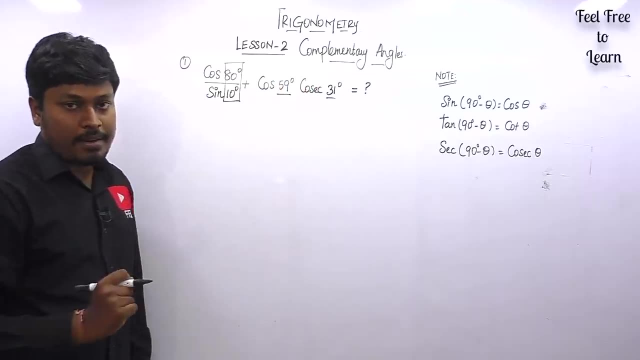 angle. Similarly, you can see here it is 59 degree and 31 degree. So sum of two angle is 90 degree. So we are saying the complete question is based on a complementary angle. So let me do one thing. 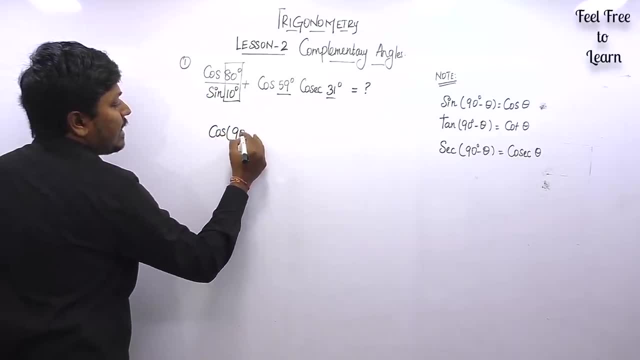 The same numerator can be written as cos of 90 degree minus 10 degree, because 90 minus 10 will be 80. So we can say cos of 90 minus 10 degree divided by. So keep the denominator as it is. 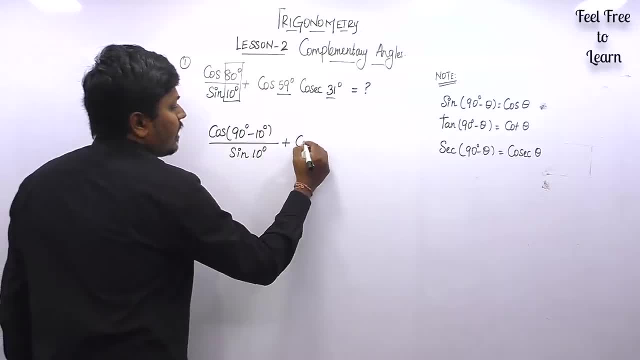 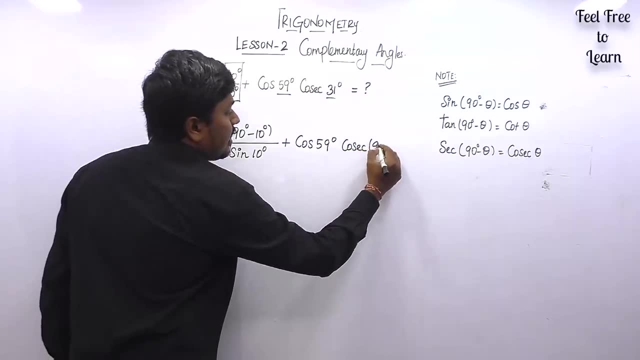 sine 10 degree, So plus cos 59 degree, I am going to write cos 59 as it is, and cosecant 31 degree can be written as cosecant 90 minus 59 degree. So friends got it. So I am converting the. numerator as 90 minus 10 degree. So I am converting the numerator as 90 minus 10 degree. So I am writing a common denominator: cos 90 minus teta and cos cos f of 30 into 50. So if you understand, 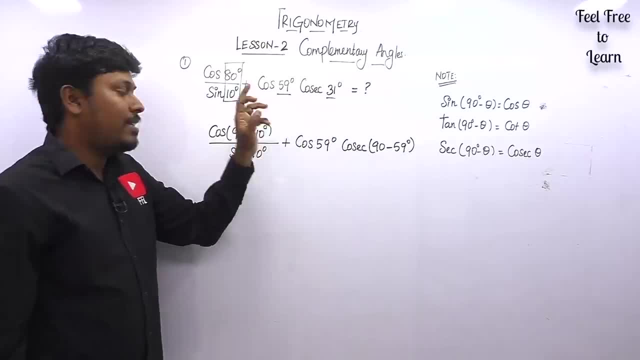 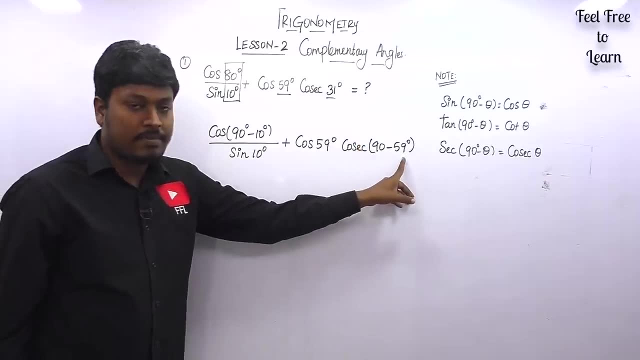 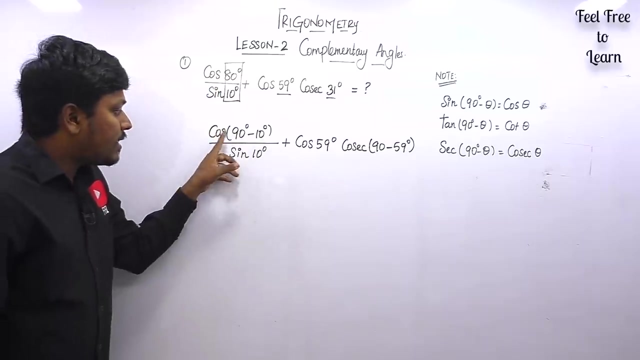 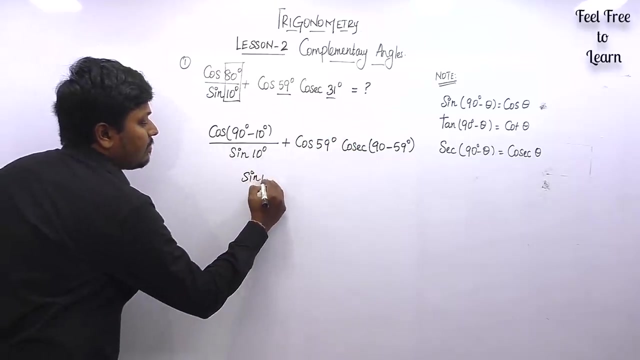 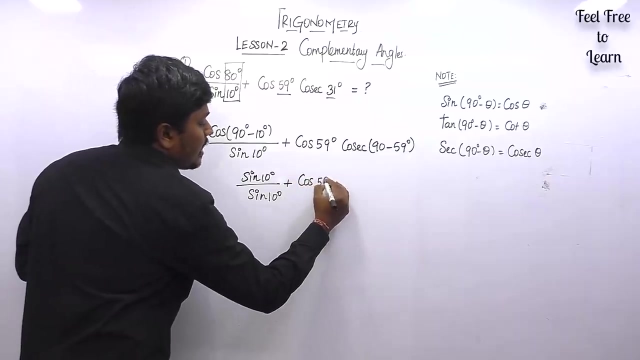 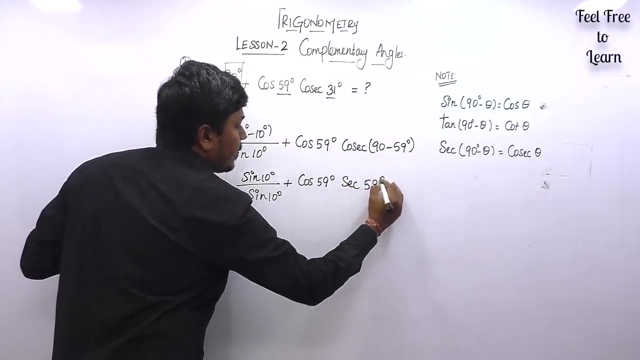 what I am saying, it is fixed. So if you have this kind of a equation already of viscosity and degree, So plus cos 59 degree, cosecant 90 minus theta, cosecant 90 minus theta will be secant theta, So secant 59 degree. So here we can cancel time theta and sine 10 degree and similarly cos. 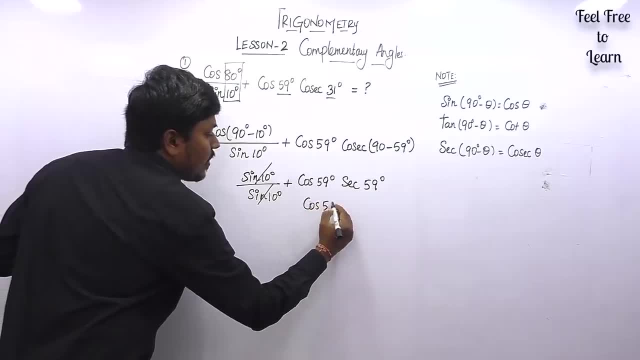 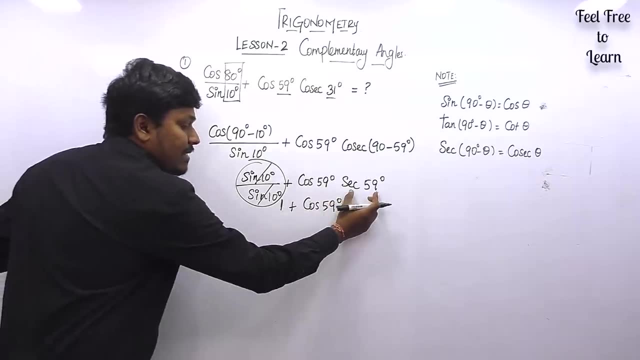 59 into secant 59. So this can be written as cos 59 degree. here we got the complete expression as 1.. So 1 plus cos 59 degree and secant will be 1 by cos theta. So 1 divided by cos 59 degree. 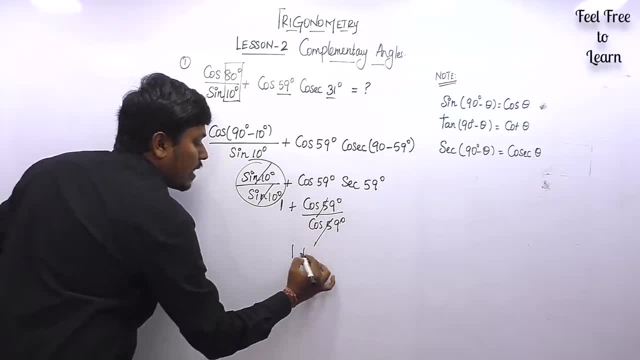 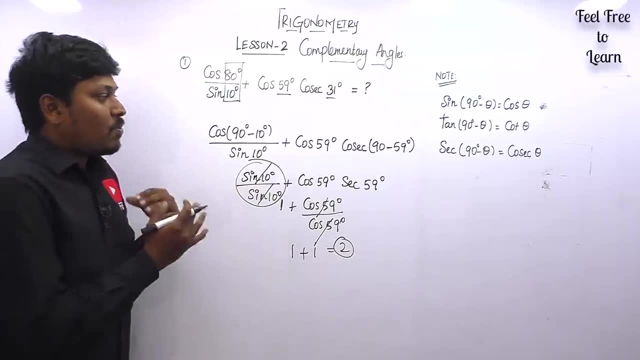 So similarly, we can cancel cos and cos. So we got 1 plus 1 is equals to 2.. So finally, answer for this question is 2.. Friends got it First. what you guys have to do First you need to check. 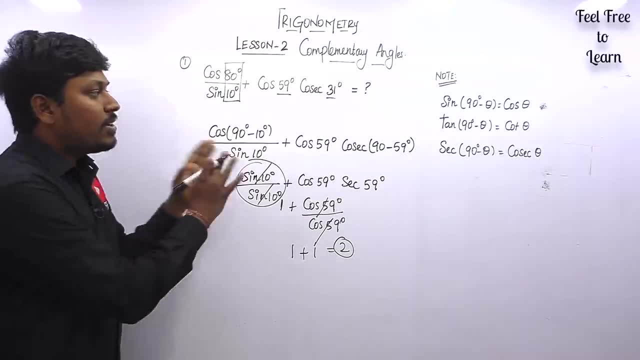 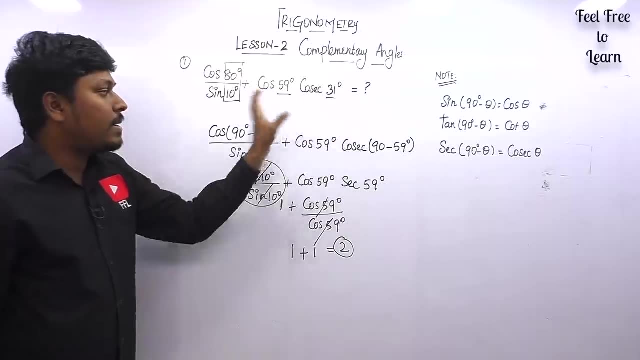 whether the question is a complementary angle or not. We found the given question as a complementary angle because 2 angle sum is 90 degree. Similarly, 2 angle sum is 90 degree, So we decide the complete question as a complementary angle. Step number 2, we convert cos theta into cos of 90. 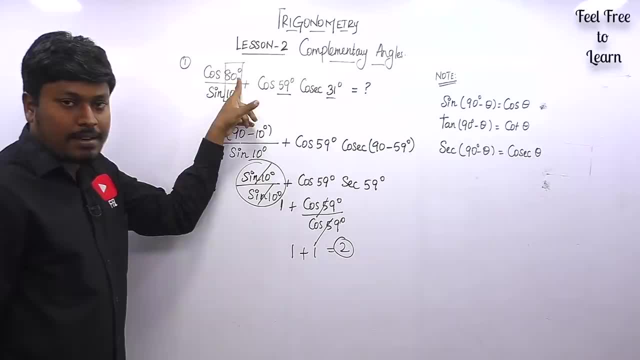 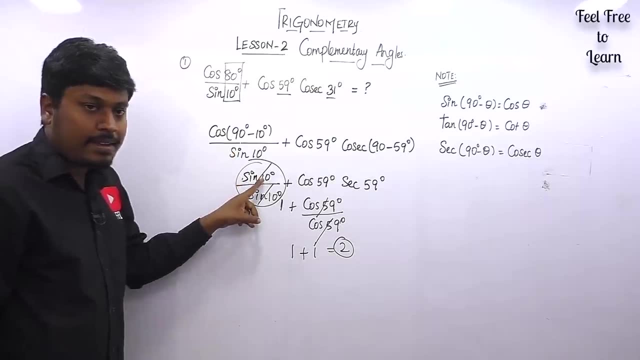 minus something. So cos 90 minus 10 will be again 80 degree. So we are writing this 80 degree as cos 90 minus theta. So cos 90 minus theta will be sine theta, that is sine 10 degree. So sine 10 by sine 10,. 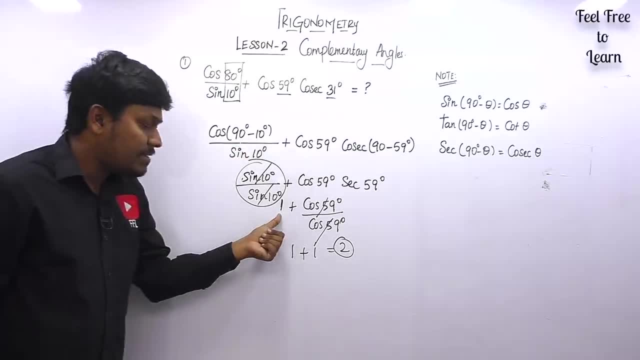 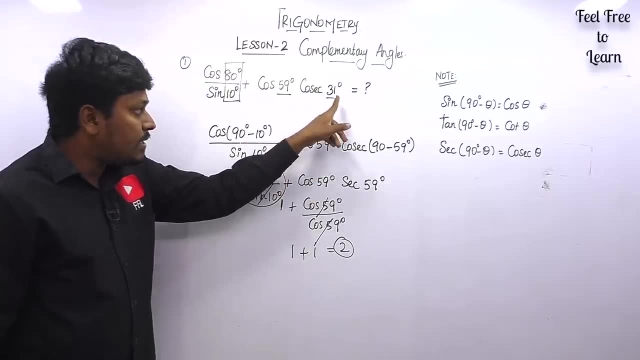 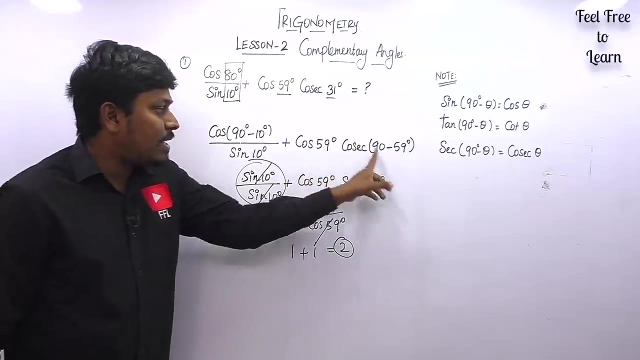 we can cancel both the term and we got the first expression. we got answer as 1.. Second expression: so keeping the first term as it is cos 59 degree. converting the second term, cosecant 31 degree, as cosecant 90 degree minus 59 degree, because 90 minus 59 will be 31.. So cosecant 90 minus. 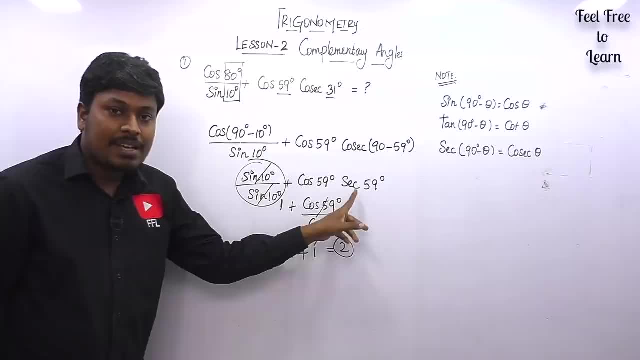 theta will be secant theta, that is secant, 59 degree. So secant can be written as 1 by cos, So 1 divided by 59 degree. So finally cos of 59,, cos of 59, we can cancel both the. 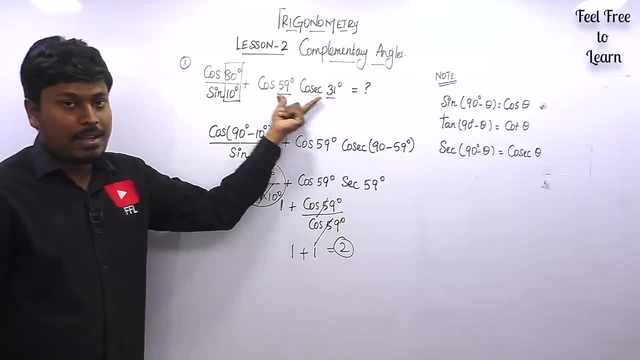 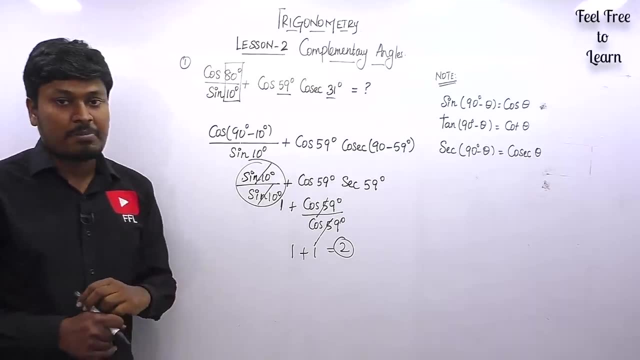 terms again and the second expression also. we got an answer as: 1.. First expression: 1 plus second expression 1.. So 1 plus 1 will be 2.. So this will be the answer for question number 1.. So beginners, you will feel little bit odd, but if you just watch the complete 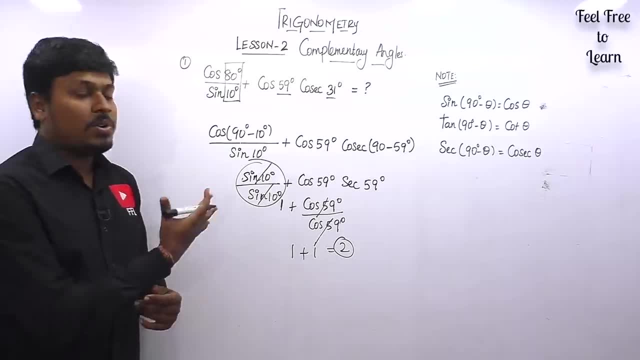 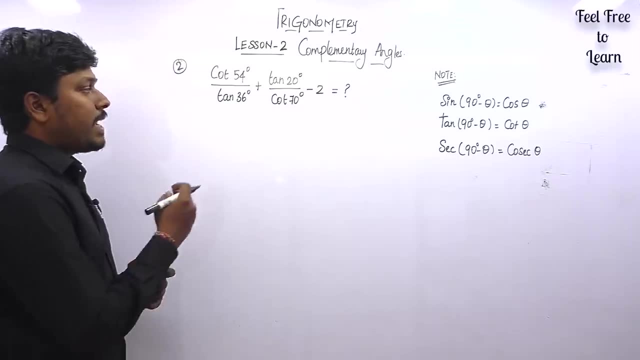 video. definitely you can able to solve all the question on the top of the screen. So let us start with complementary angles. Question number 2.. So cot 54 degree divided by tan 36 degree plus tan 20 degree, divided by cot 70 degree minus 2, is equal to question mark. 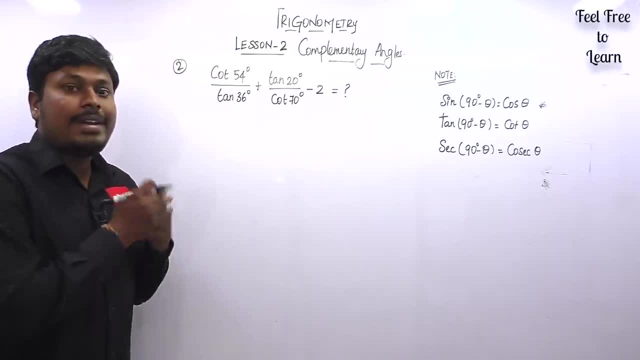 So just check whether it is a complementary angle or not. Yeah, it is a complementary angle because sum of two angles here, 54 degree, 36 degree, So sum of two angles is 90 degree. So we can say the two angle is a complementary angle. So, similarly, 20 degree, 70 degree again. 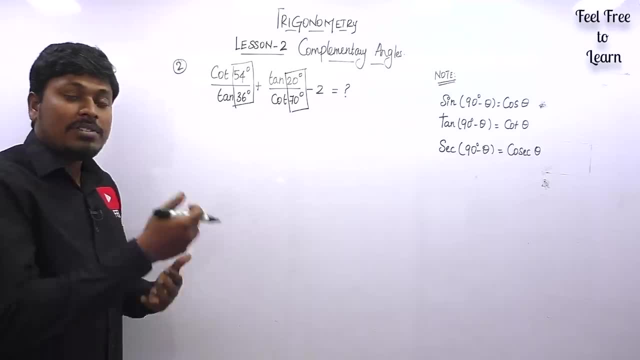 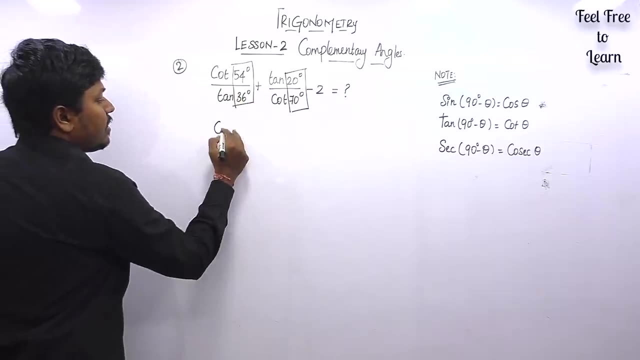 it is a complementary angle. So if it is a complementary angle, it is a complementary angle. What is your step number 2?? You need to convert either numerator part or a denominator part. It is completely your wish, right. So cot can be written as cot of 90 degree minus 36. 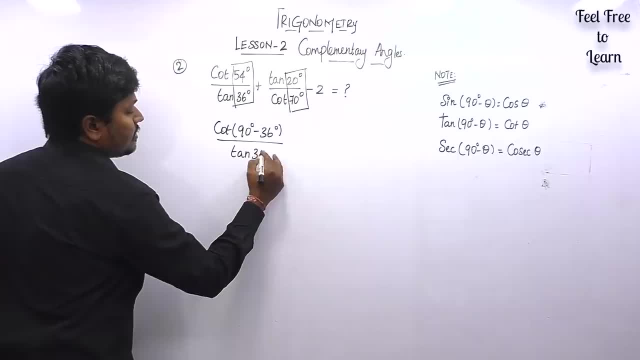 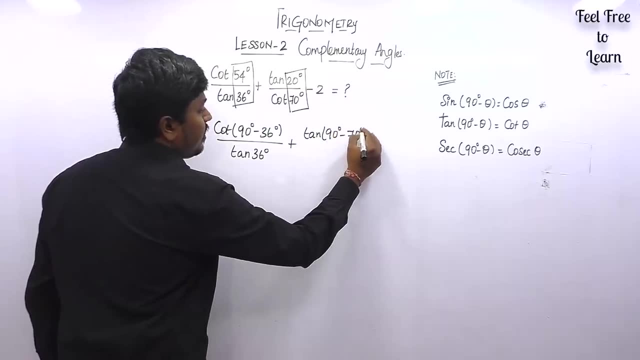 degree divided by the denominator, that is tan, 36 degree. Got it? So similarly, tan 20 degree can be written as tan of 90 degree minus 70 degree. divided by cot, 70 degree minus 2 is equal to question mark, Got it? 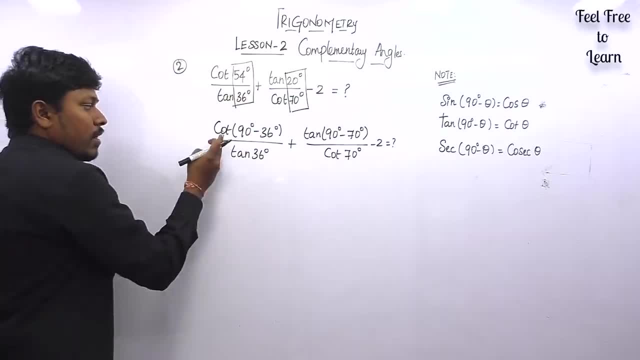 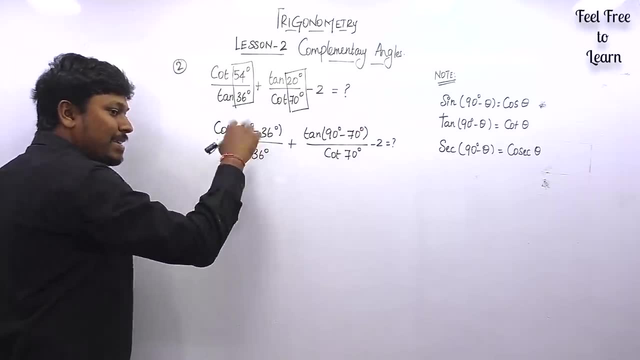 It will be 20.. Similarly, 90 minus 36 will be 54. Now cot 90 minus theta- What is cot 90 minus theta? will be tan theta. So cot 90 minus 36 will be tan 36 degree, So tan. 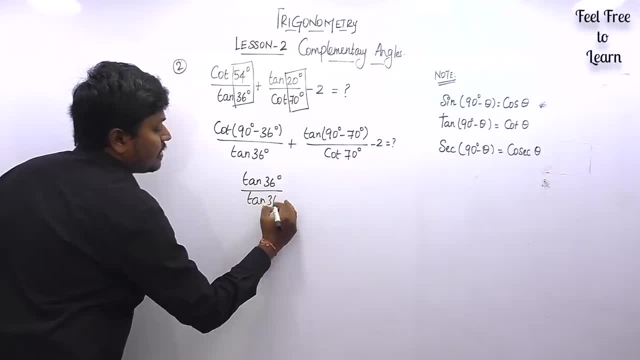 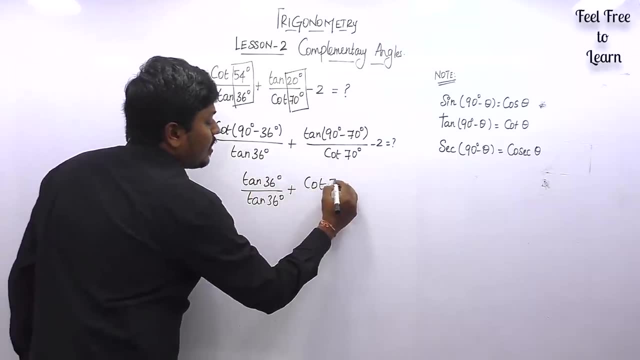 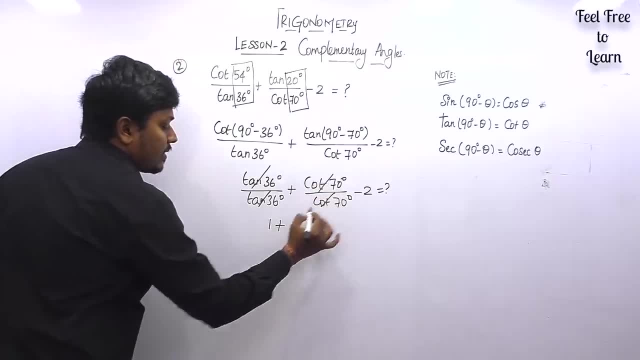 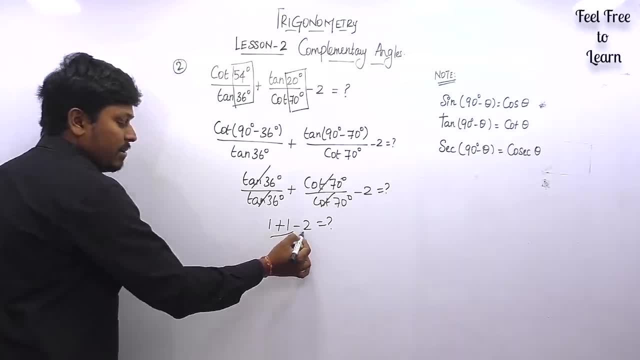 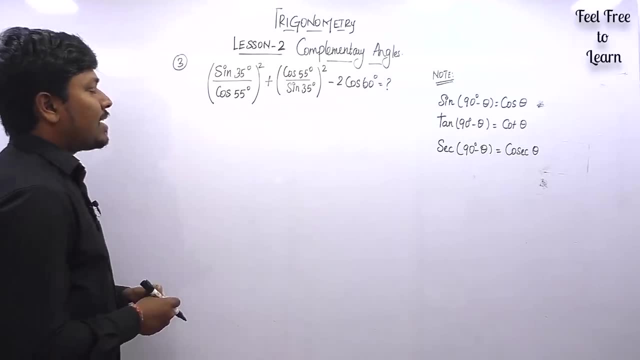 mark. So 1 plus 1 will be 2.. So 2 minus 2 will be 0.. So finally we got an answer for question number 2, that is 0.. Question number 3.. So sin, 35 degree divided by cos. 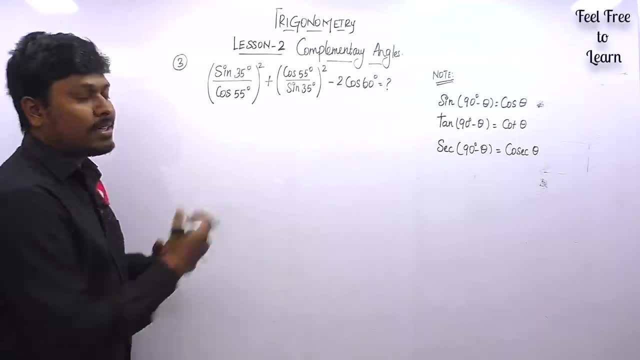 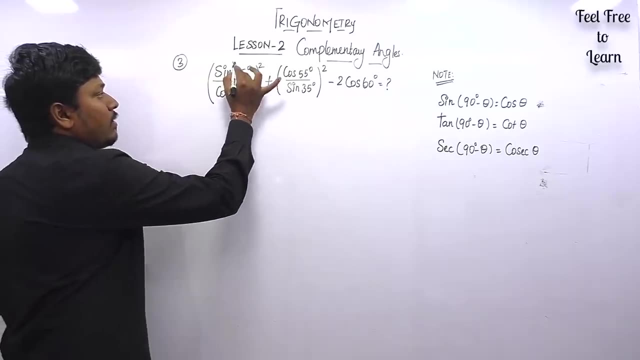 55 degree the whole square. So similarly, second expression and third expression. So first see whether it is a complementary angle or not. important question right. See here: 35 degree and 55 degree. Once you add both, the angle resultant will be 90 degree. So 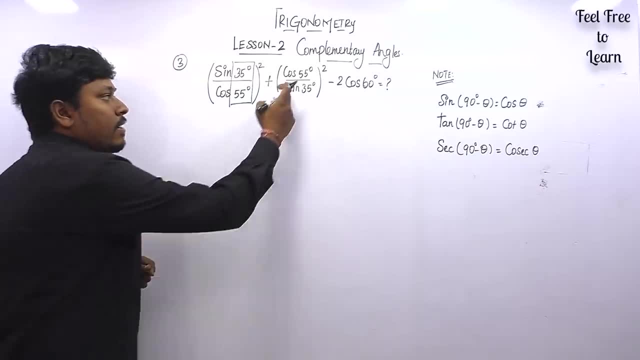 we can say the first expression is a complementary angle. Second, cos 55 sin 35 again, if you add the two angle then the resultant will be 90 degree. So we can say this expression is also a complementary angle. But when you look at the last term, 2 cos 60 degree, whether it 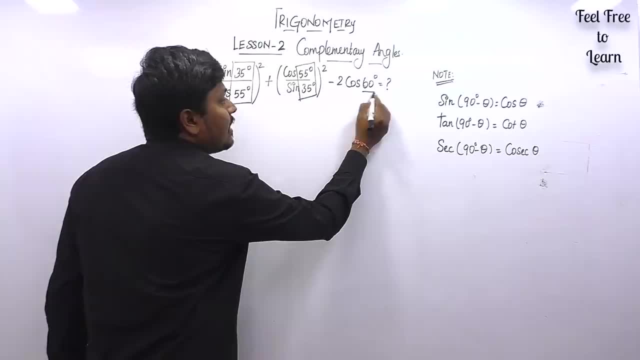 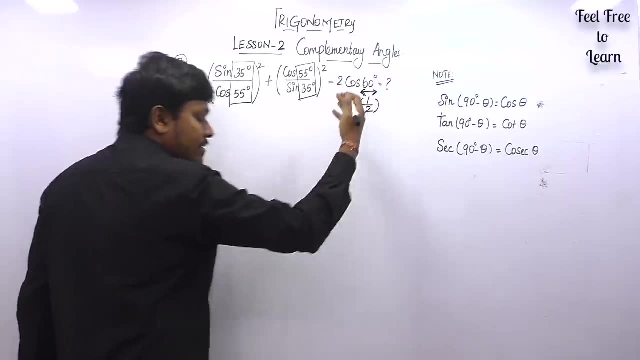 is a complementary angle. no, it is not a complementary angle. It is a direct trigonometrical value, What is called as cos 60?? So cos 60 will be 1 by 2.. So, according to lesson number 1, we have learnt already, right? If? 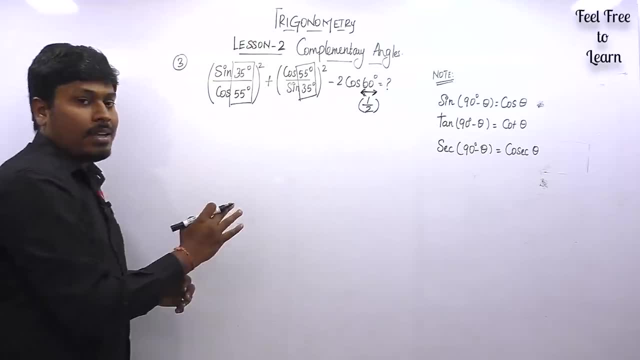 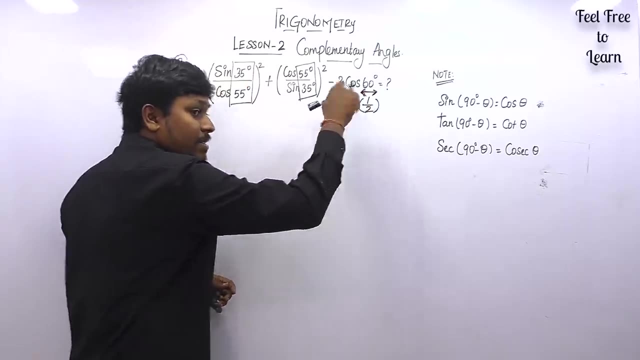 it is a direct trigonometry ratio. you can substitute the value If it is a complementary angle. we do not have a trigonometrical ratio as sin 35 degree, But we have what is cos 60 degree, according to the table chart which I have taught you on lesson number 1.. So 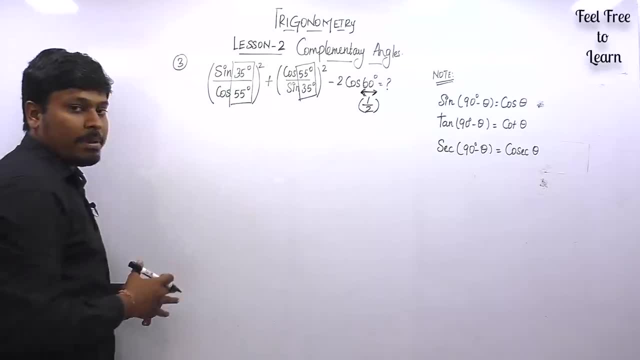 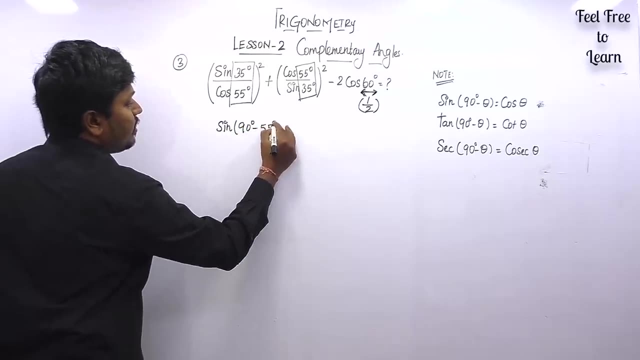 cos 60 degree will be 1 by 2.. So remaining two expression is a complementary angle. So let me convert this So this can be written as sin 90 degree minus 55 degree, So divided by the denominator cos 55 degree, So plus. similarly, cos 90 degree minus 35. 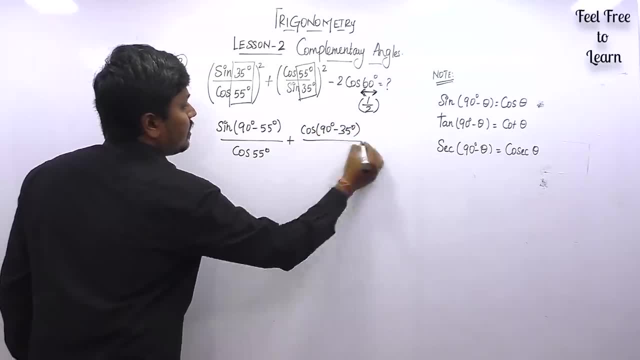 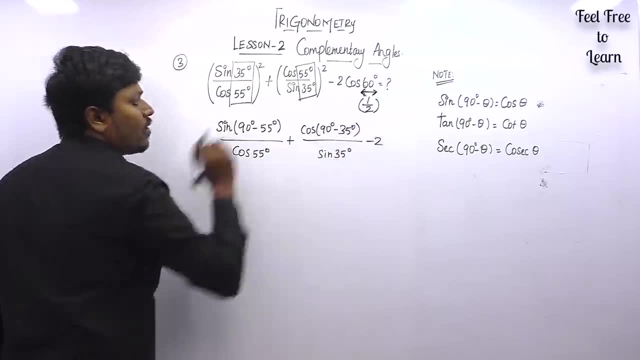 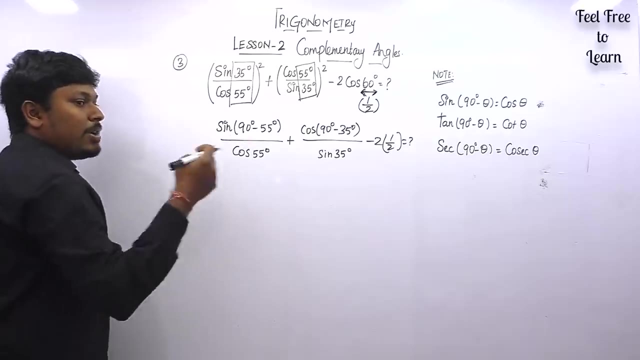 degree divided by sin, 35 degree. So plus- sorry, minus- of 2 into. we know that cos 60 degree will be 1 by 2.. So 1 divided by 2 equal to question mark. friends got it. So sin 90 minus theta will be cos theta. So here we have 55 degree. So cos 55 degree. 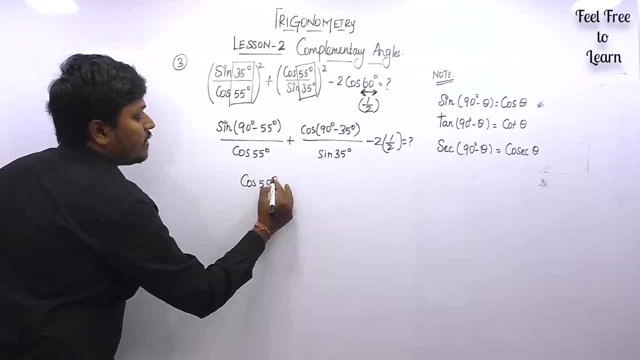 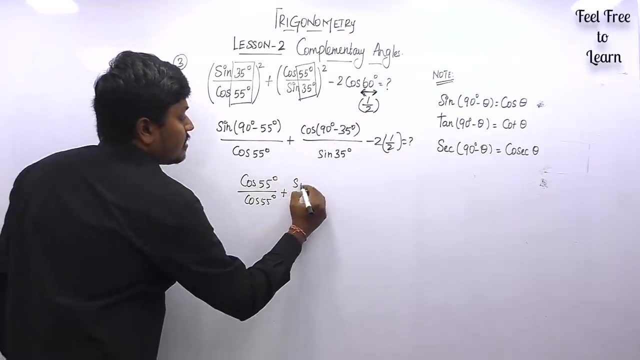 divided by cos 55 degree, we can write cos theta plus plus, minus of sin theta. So here, divided by cos 55 degree, So plus cos 90 minus theta will be sin theta, So sin 35 degree. divided by sin 35 degree, So minus, we can cancel 2 and 2.. So finally we got minus. 1 is equal to question. 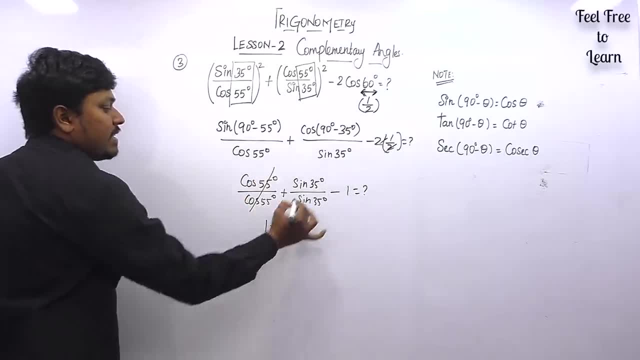 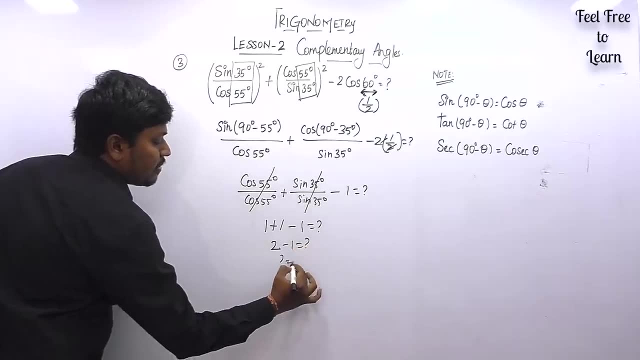 mark. So cos 55, cos 55 will be 1 sin 35, sin 35 will be again 1.. So minus 1 is equal to question mark. So 2 minus 1 is equal to question mark. So question mark is equal to 1.. So finally, 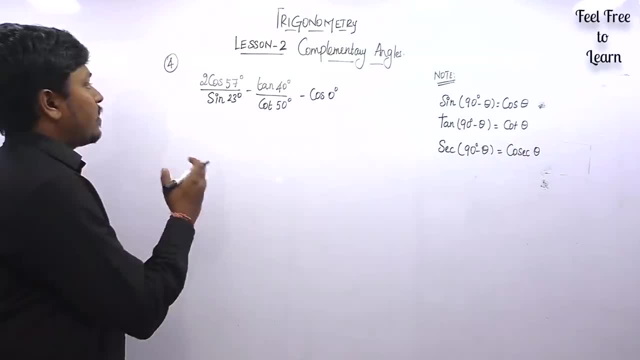 for question number 3, we got an answer as: 1. Question number 4.. So 2 cos 57 degree divided by sin 23.. So minus tan 40 by cot 50 minus cos 0 degree is equal to question mark. So listen here. 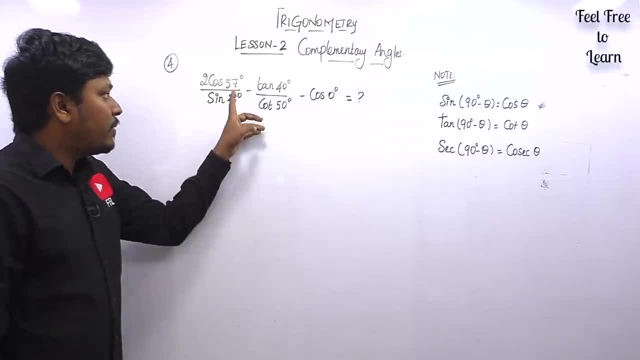 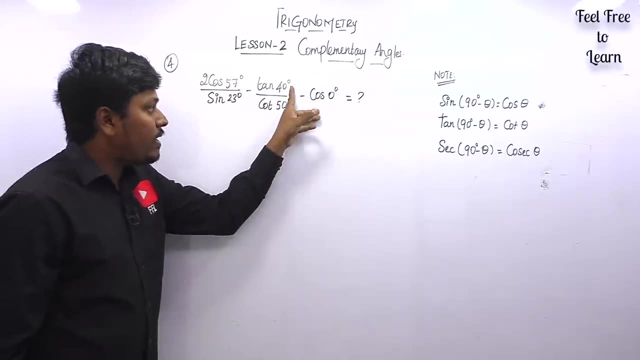 whether it is a complementary angle or not. Yeah, it is a complementary angle because 57, 23.. If you add both, the angle resultant will be 90 degree. So it is a complementary angle. So, similarly, 40 degree, 50 degree, again it is a complementary angle, but the last value is cos 0 degree. 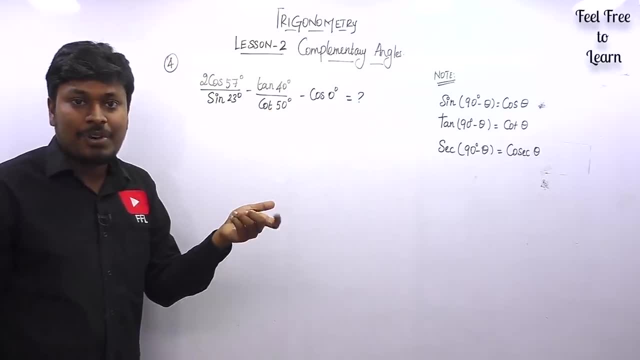 Whether it is a complementary angle. no, it is a direct trigonometry ratio. What is cos 0 degree? Cos 0 degree will be 1.. So, according to the table chart, we already know that cos 0 degree is 1,. 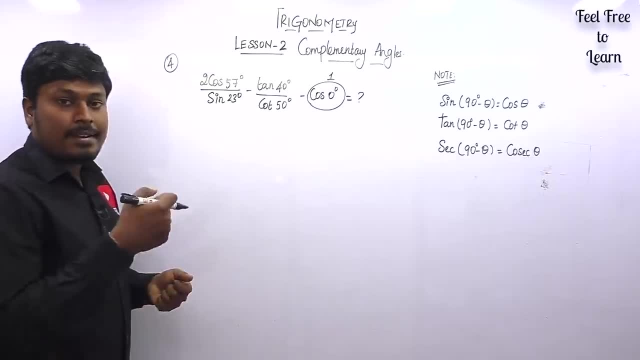 cos 90 degree is 0, sin 0 degree is 0, sin 90 degree is equal to 1.. So these are the stuff we learned in lesson number 1.. It is a direct trigonometry ratio. Got it. So first expression: 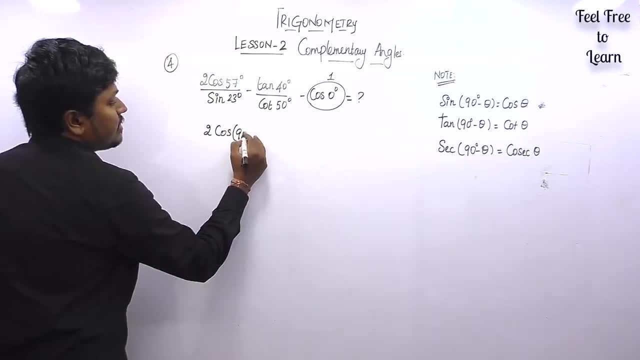 2 into cos 57 degree can be written as 90 degree minus 23 degree. So divided by sin 23 degree we can keep it as 1.. So this is the first expression. So this is the first expression. 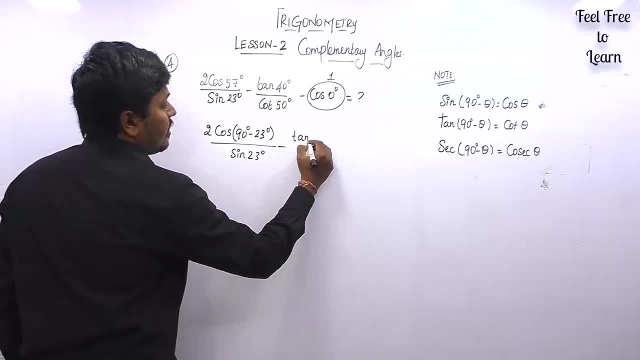 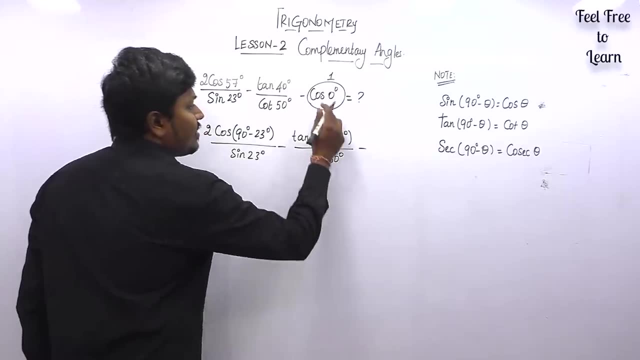 So it is minus of tan. 40 degree can be written as tan of 90 degree minus 50 degree. So divided by cot 50 degree. So minus cos 0 degree will be 1.. So minus 1 is equal to question mark. 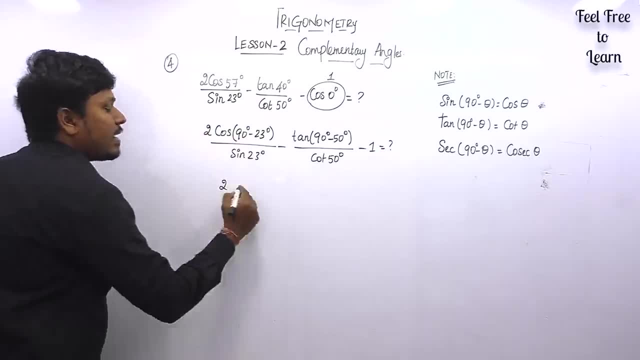 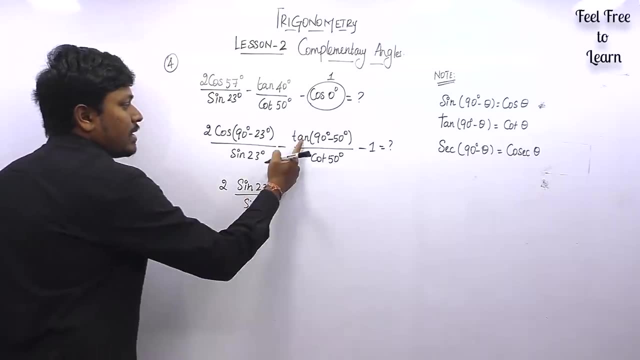 So 2 into cos 90 minus theta will be sin theta, So sin 23 degree divided by again sin 23 degree, So minus of tan 90 minus theta will be cot theta, that is cot 50 degree divided by again. 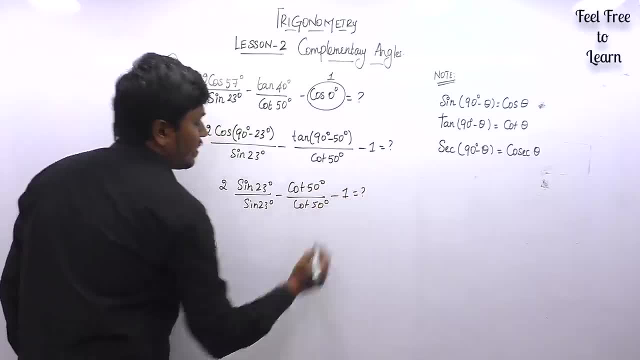 again cot 50 degree. So minus 1 is equal to question mark. So you can cancel sin and sin cos and cot, sorry, cot and cot. So finally we got 2 minus 1. minus 1 is equal to question mark. 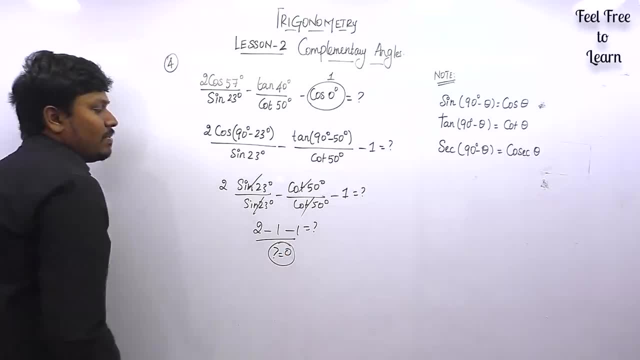 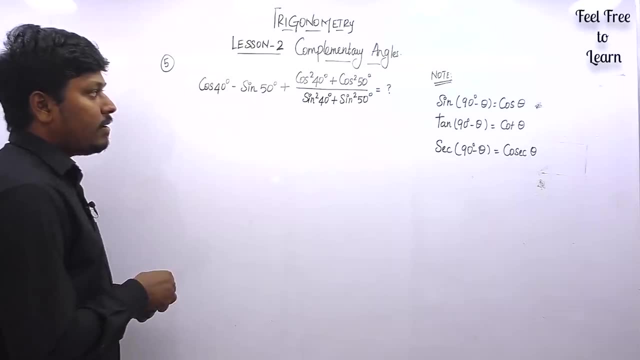 So 2 minus 2 will be 0.. So 0 will be the answer for question number 4.. Question number 5.. So cos 40 degree minus sin, 50 degree. So plus cos square 40 degree plus cos. 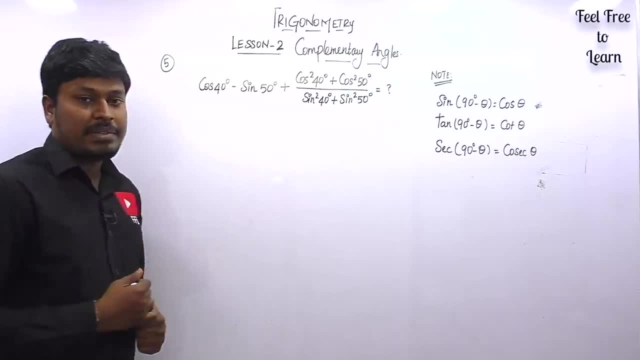 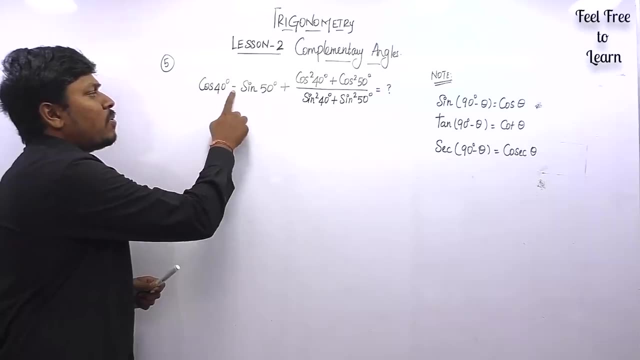 square 50. sin square 40 plus sin square 50 is equals to question mark. Just see here whether it is a complementary angle. it is complementary angle because 40, 50, sum of 2- you do not want to care about negative symbol right- 40 and 50. So sum of 2 angle is 90 degree. So similarly 40- 50. 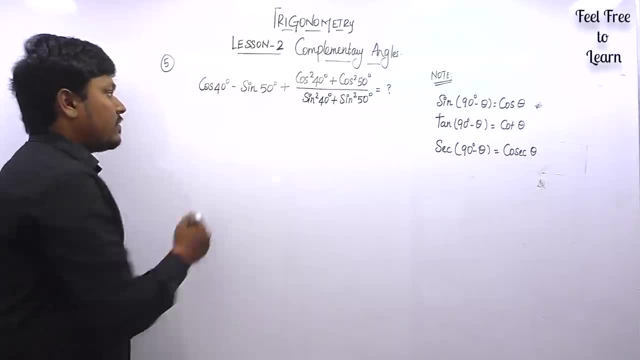 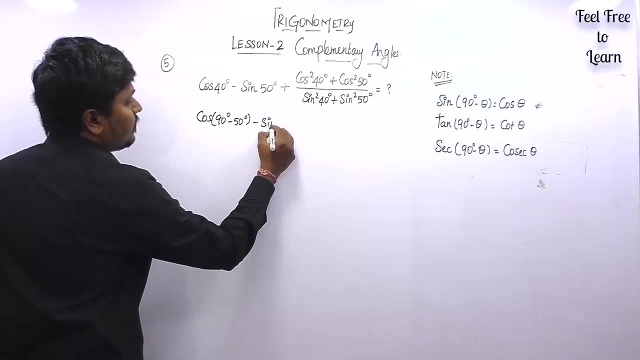 complementary pair, So 40, 50, again complementary angle. So first let me convert this as cos of 90 degree minus 50 degree, So minus of sin 50 degree. So plus sin 50 degree. So plus sin 50 degree, So minus of sin 50 degree. So plus sin 50 degree. So 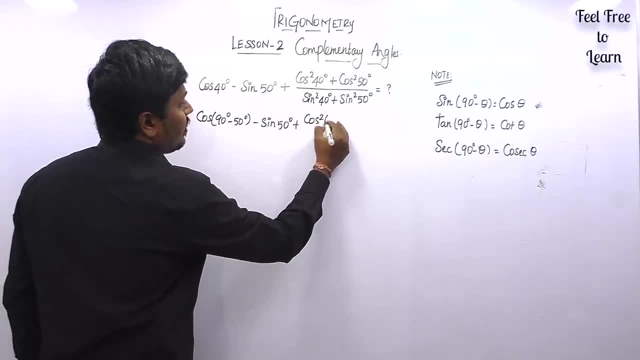 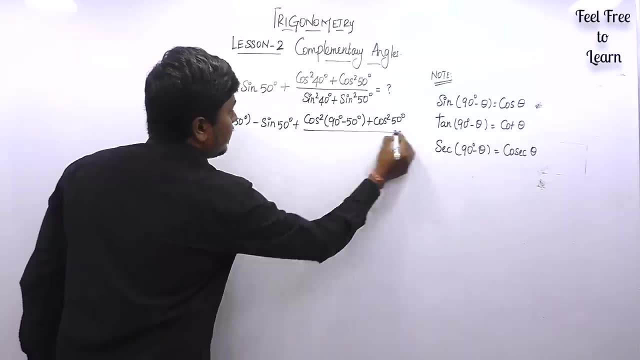 and we convert any one expression right. So this can be written as cos square 90 degree minus 50 degree, So plus cos square 50 degree. So divided by so sin square 90 degree minus 50 degree, So plus sin square 50 degree, is equals to question mark. So here cos 90 minus theta. 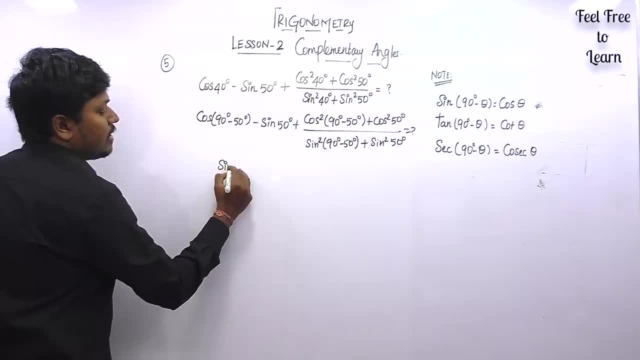 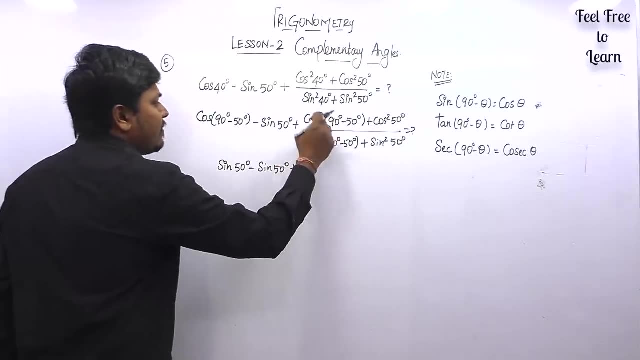 So cos 90 minus theta will be sin theta. that is, sin 50 degree minus of again sin 50 degree, So plus. so cos 90 minor, leave the square right. So cos 90 minus theta will be sin theta. So 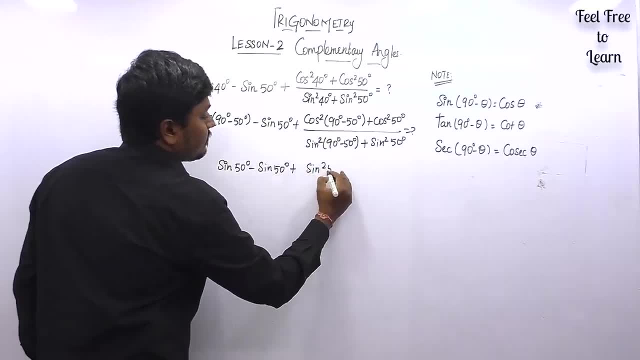 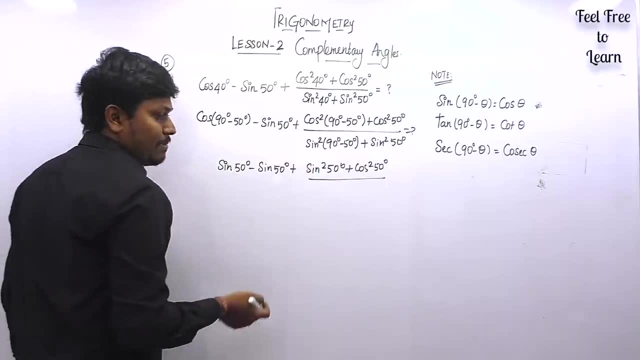 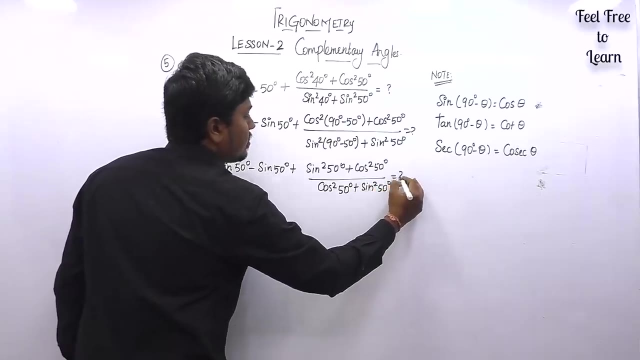 this can be written as sin square 50 degree. So sin square 50 degree plus cos square 50 degree. divided by again sin 90 minus theta will be cos theta. So cos square 50 degree plus sin square 50 degree is equals to question mark. So here you can cancel sin 50 degree minus sin 50 degree. 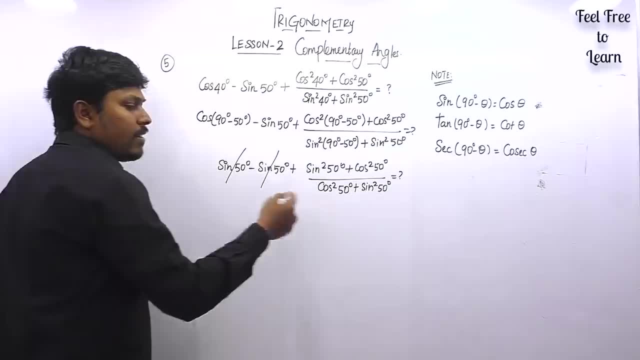 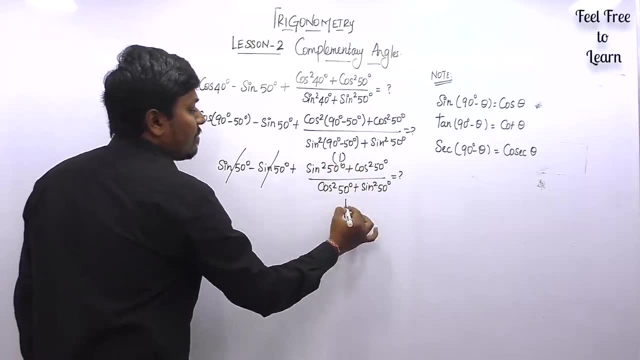 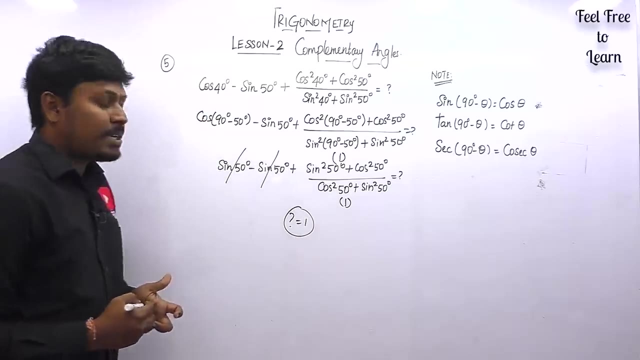 resultant will be 0.. Either you can cancel directly here or otherwise. we know sin theta plus cos theta, Sin square theta plus cos square theta is equal to 1.. So numerator 1, denominator 1.. So 1 divided by 1 will be 1.. So question mark is equal to 1.. So finally answer for question number. 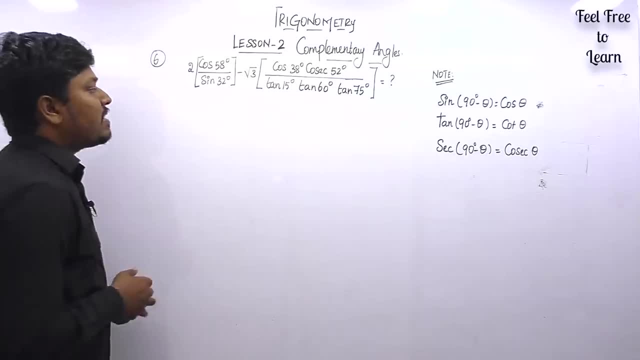 5, where question mark is equals to 1. Question number 6.. So 2 into cos 58, divided by sin 32 again, if you add both the angles then the resultant will be 90 degree, So we can say it is a complementary angle. 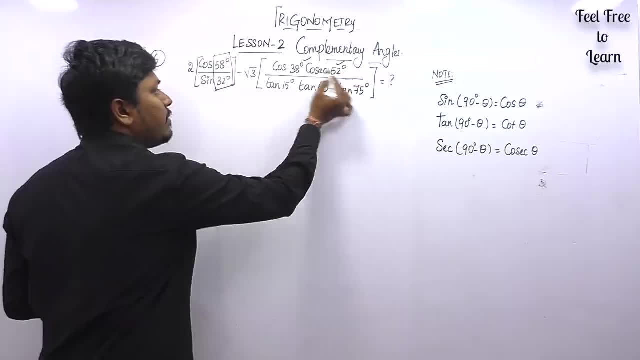 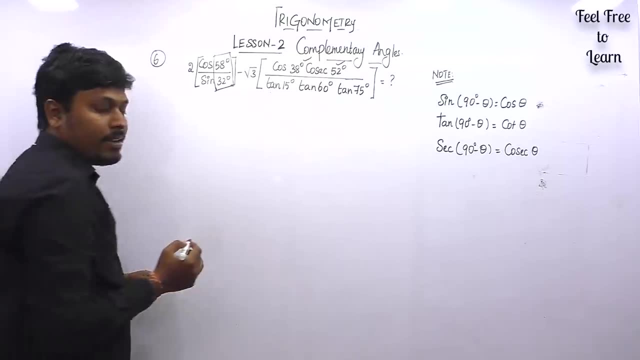 So similarly, cos 38 degree, cos 52 degree, again both the angle is a complementary angle. So look at the denominator tan 15 degree, tan 60 degree, tan 75 degree, and here we can surely say tan 60 degree is a direct denominator ratio, because according to table chart we: 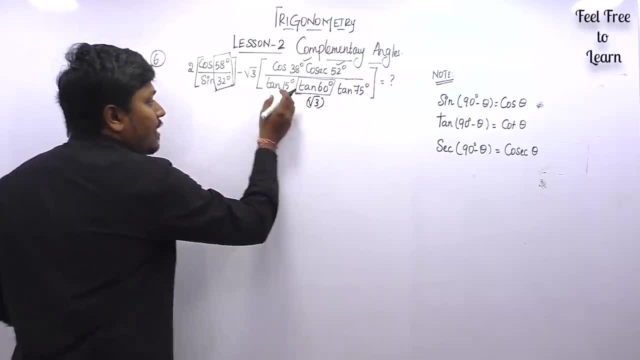 know that tan 60 degree will be root 3 and the remaining tan 15 degree and tan 75 degree. So 75 degree and 15 degree will be a complementary angle. So we can say these two are a complementary angle. 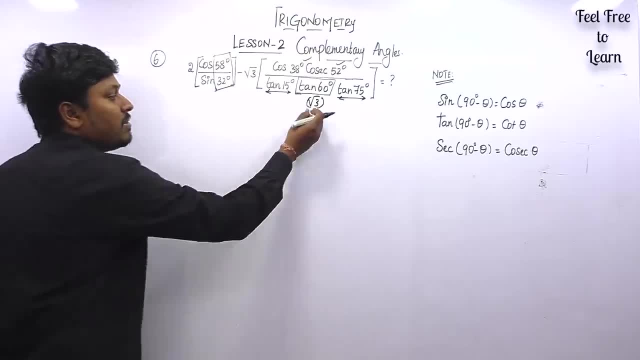 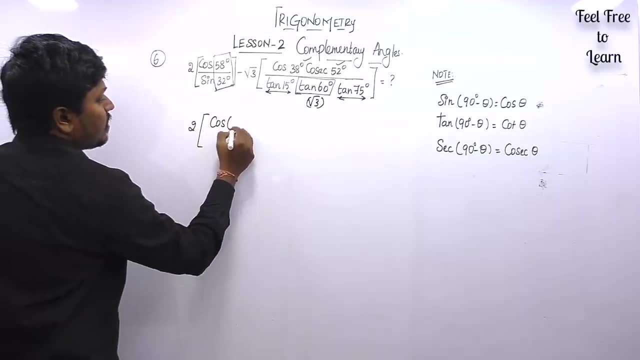 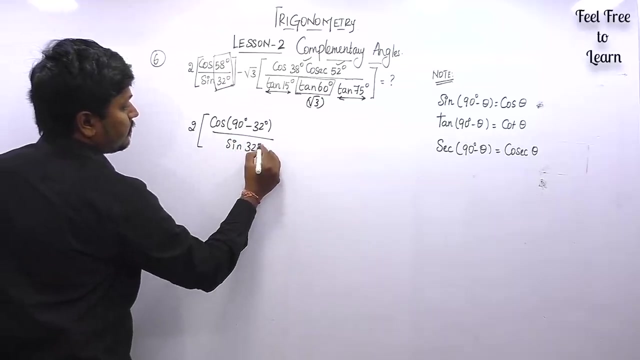 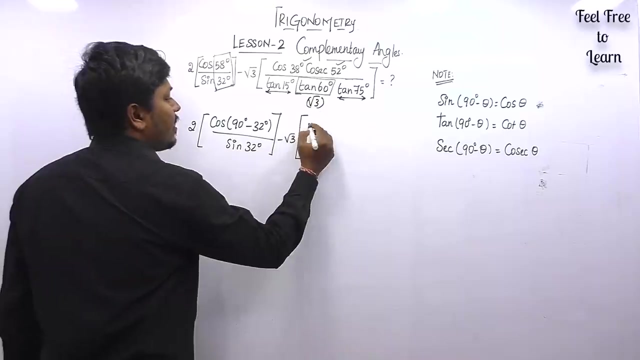 So we can say that is the trying to measure, So we can say that this is the AT angle right. So this is the tentative angle. governors, slope angle, cones angle, or the conditions of Courbet, all those is a complementary angle. So you look, the tan 60 degree angle is a決. �. 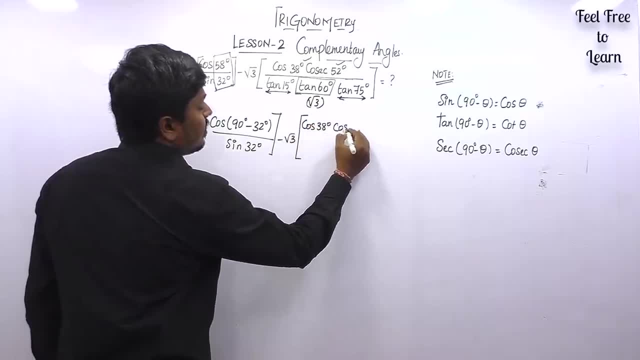 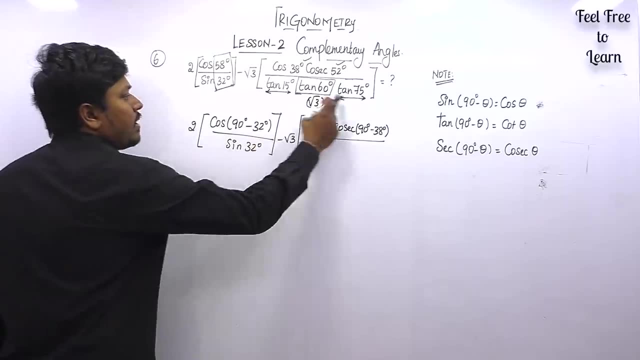 dressed at 42 degree in franches given value. but the tan 60 degree is a direct geometry value, That is root 3.. So now let me do one thing. we can write this as 2 into cos 57 degree and the cosecant 90 degree minus 38 degree. so divided by so tan 15 degree, tan 75 degree. 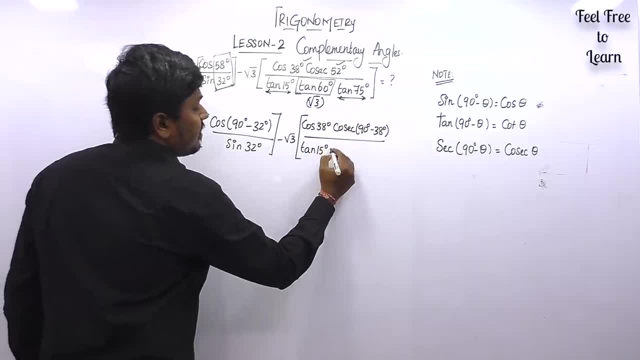 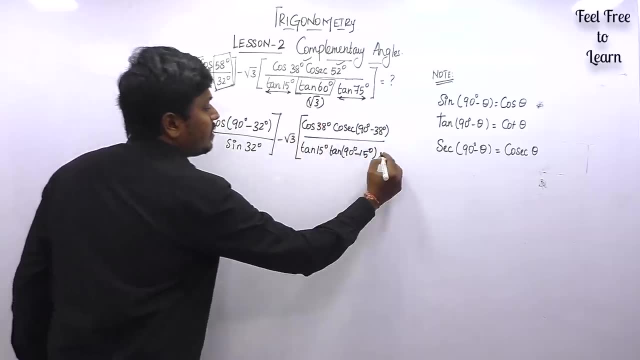 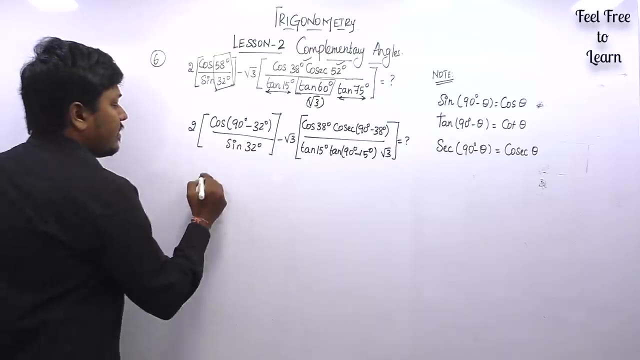 so we can write this as tan 15 degree and this tan 75 can be written as tan of minus 15 degree and tan 60 degree will be root 3, so into root 3 is equals to question mark. So cos 90 minus theta will be sine theta. so 2 into sine 32 degree divided by sine 32. 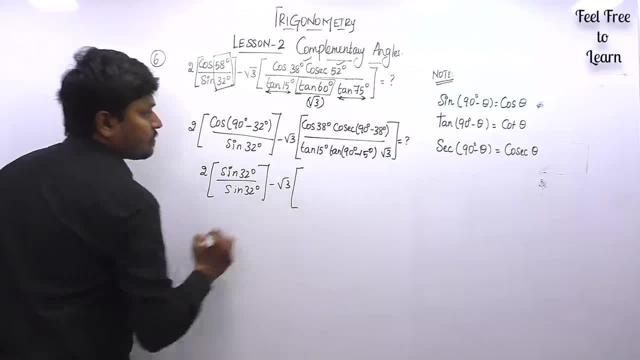 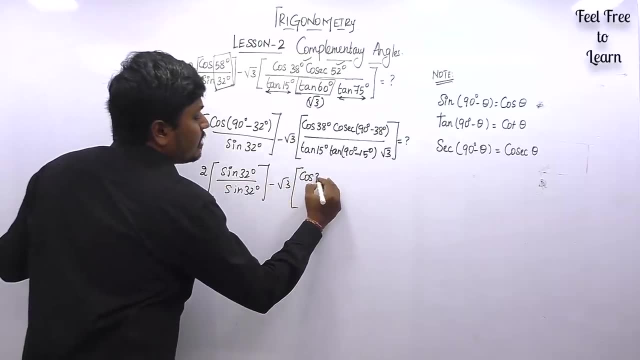 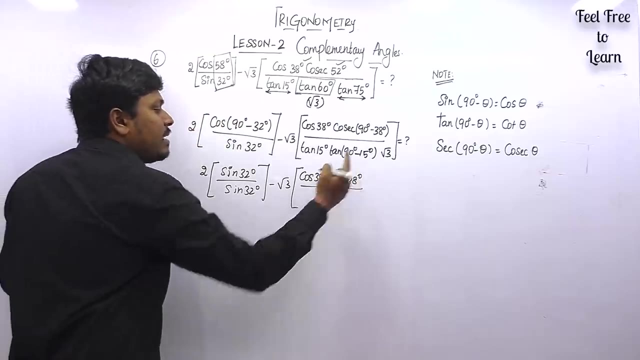 degree, so minus of root 3. into so cosecant 90 minus theta. cosecant 90 minus theta will be secant theta. so this can be written as cos 38 degree. so into secant 38 degree. divided by so tan 90 minus theta will be cot theta, so tan 15 degree. 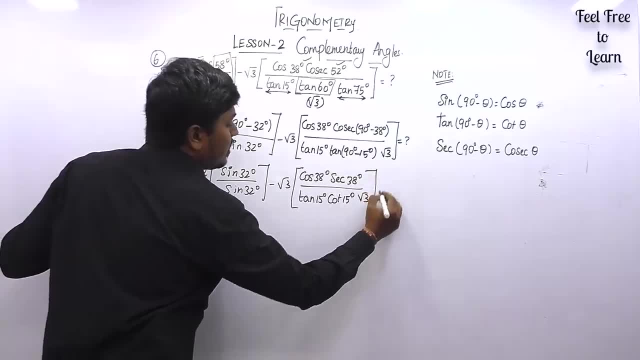 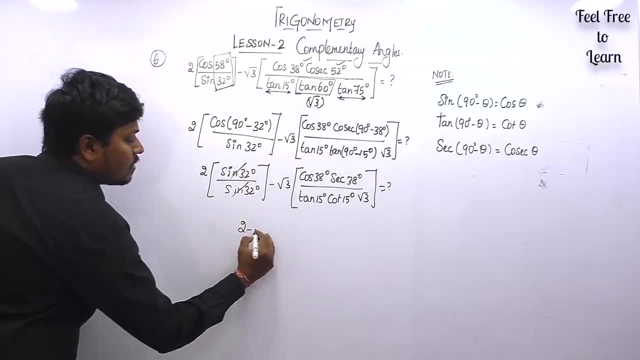 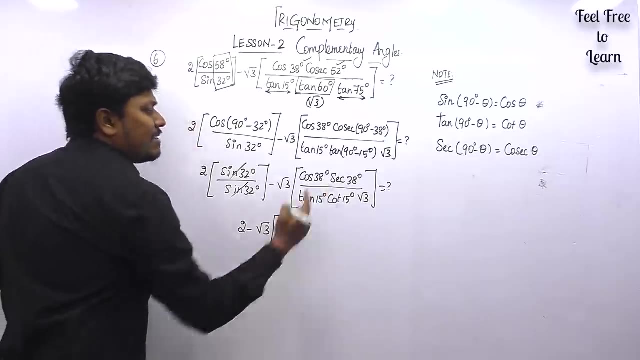 Cot 15 degree into root 3 is equals to question mark. So now 2 into we can cancel sine theta. sine theta, so first expression we got an answer as 2, so minus of root 3 into. so cos 38 degree and secant 38, we know that secant will be. 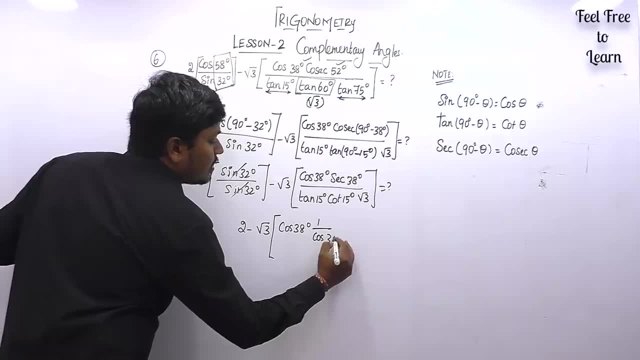 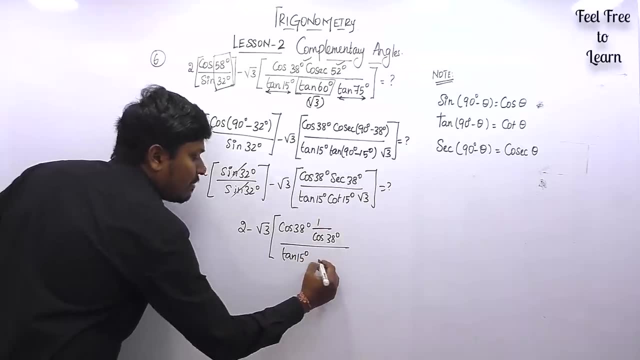 1 by cos. so secant 38 can be written as 1 divided by cos 38 degree, so divided by. similarly, tan 15 degree And cot 15 degree can be written as 1 by cos 38 degree. So this is 1 by tan. so 1 by tan 15 degree into root 3 is equals to question mark. 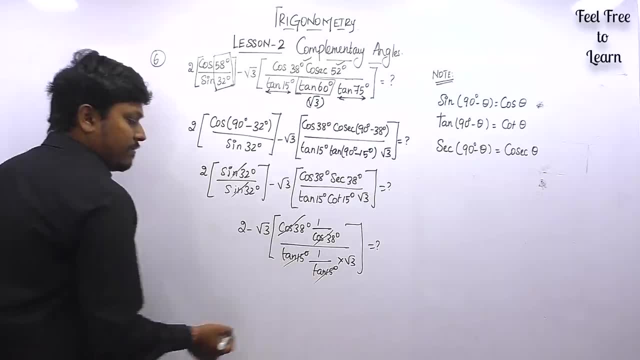 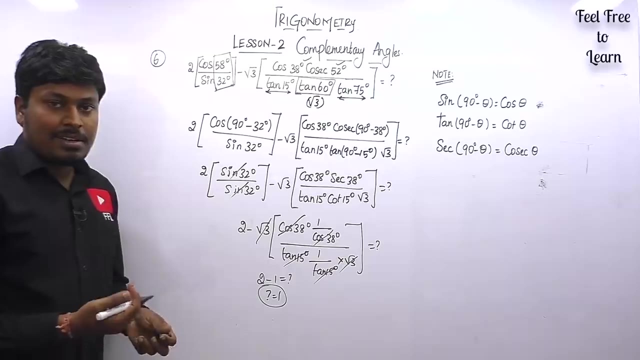 So you can cancel cos 38,, cos 38, tan 15 and tan 15.. So finally, we can cancel root 3 and root 3.. So complete second term got cancelled and resultant will be 1.. So 2 minus 1 will be 1, so question mark will be 1, that is it easiest equation. 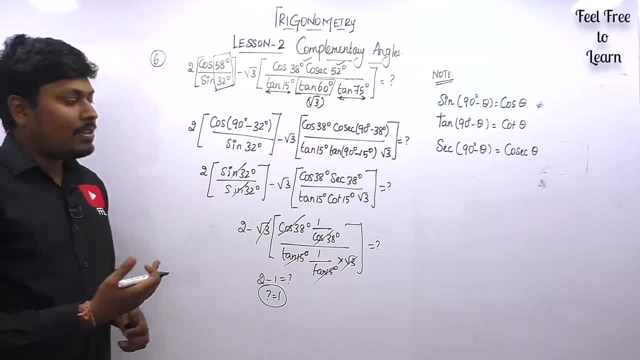 So if you practice more and more number of question, definitely trigonometry will be very easy, But you have to know some of the concepts like complementary angle, acute angle, abducer, angle right. We will be teaching on next 3 or 4 lessons. 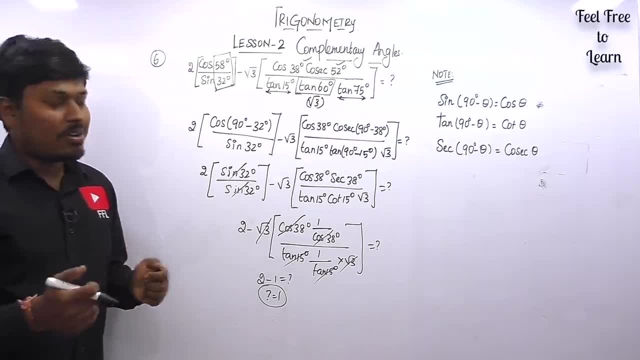 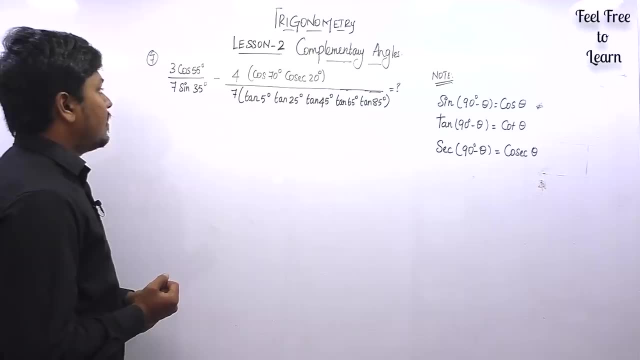 So all the concepts are important and trigonometry is the easiest topic. got it. So here, finally, we got an answer for question number 6, question mark is equal to 1.. Last 7th question: so 3 cos 55 degree divided by 35 degree, again, it is a complementary. 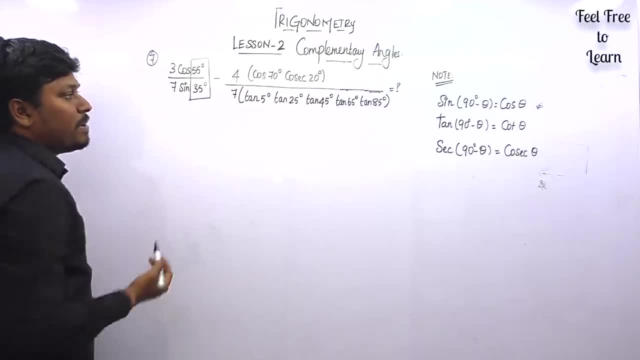 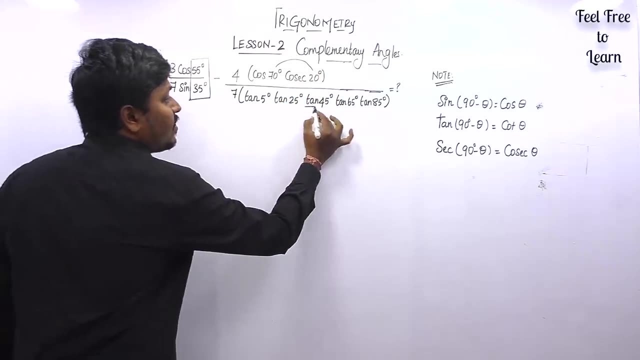 angle right. So sum of 2 angle is 90 degree, so we can say it is a complementary angle. So similarly, 70 degree, 20 degree, So complementary angle. So next will be tan 45,. listen here, it is not a complementary angle. 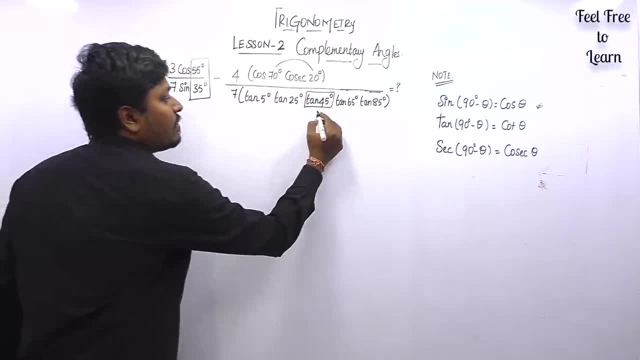 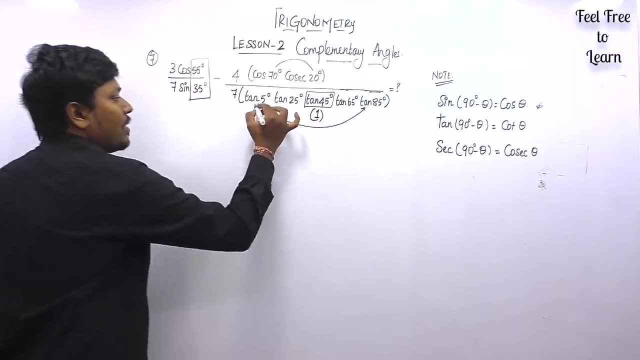 Because we know what is tan 45 degree according to table chart. So according to table chart, tan 45 degree will be 1, got it. So next will be tan. see here: tan 5 degree. tan 85 degree. 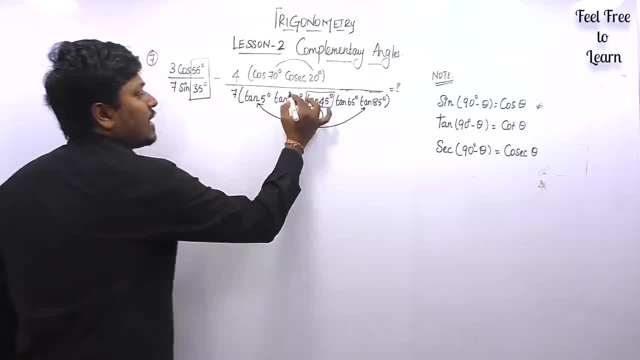 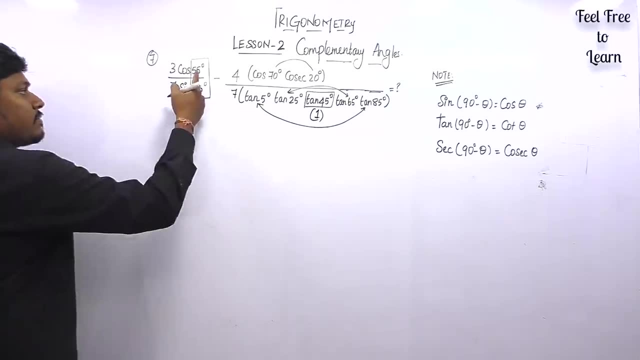 Once you add both, the angle resultant will be complementary angle 90 degree. So tan 25, tan 65 will be a complementary angle, got it? So this can be written as 3 by 7.. So cos 55.. 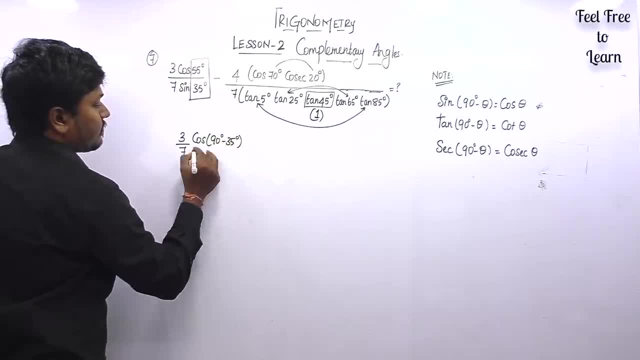 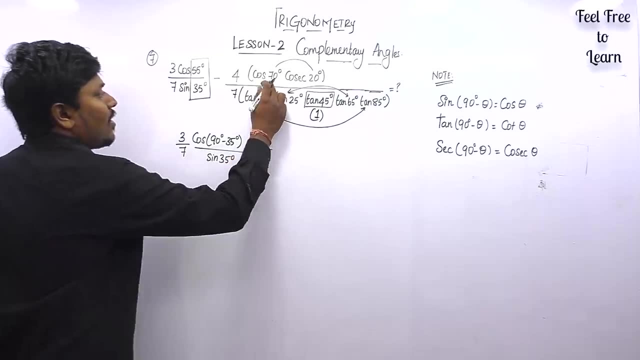 Can be written as cos 90 degree minus 35 degree, So divided by sin 35 degree, So minus of 4 by 7.. So the numerator cos 70 degree can be written as: either we can convert cos to sin or cosecant. 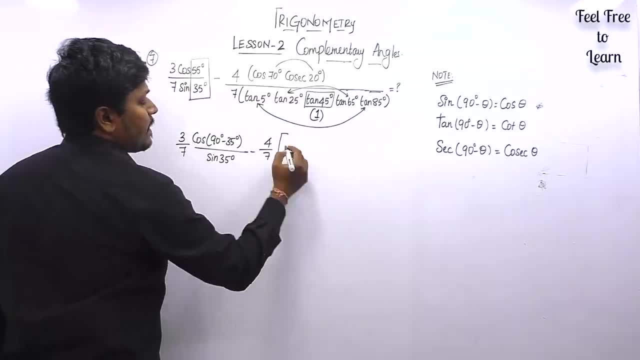 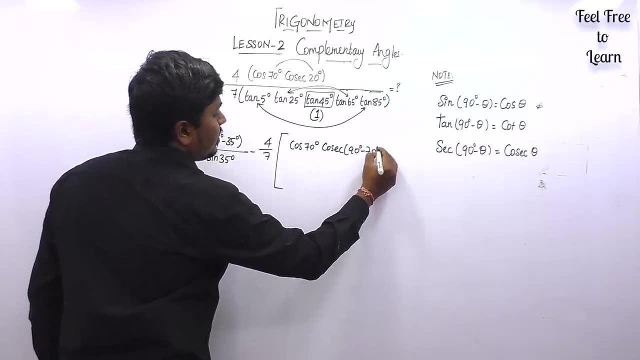 to secant. So let me do one thing. we can write this as cos 70 degree and cosecant can be written as cosecant 90 degree minus 70 degree, So divided by So tan 5 degree and tan 85 degree. 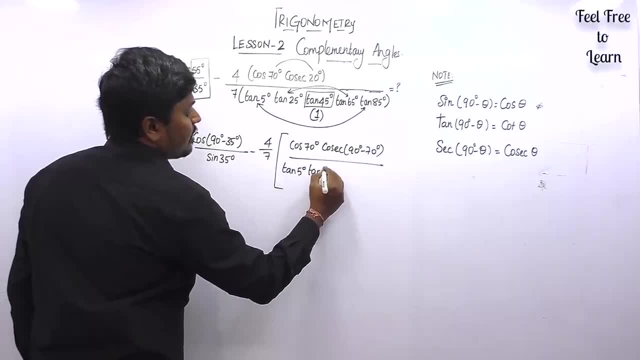 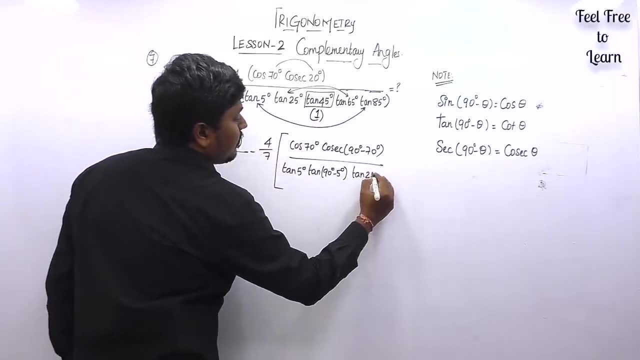 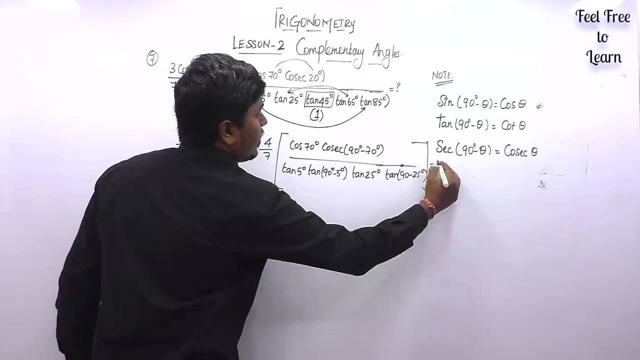 So tan 5 degree and tan 85 can be written as tan of 90 degree minus 5 degree and next tan 25, tan 65.. So tan 25 degree and tan 65 can be written as tan of 90 degree minus 25 degree equal. 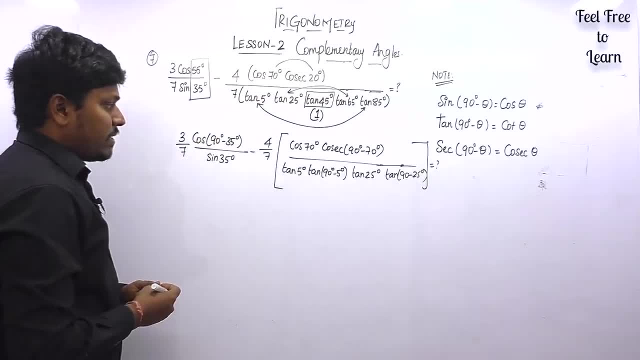 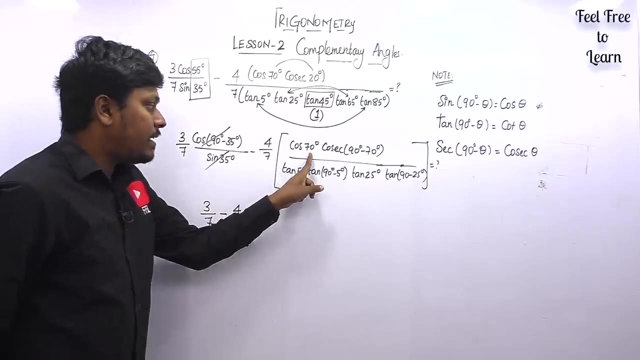 to question mark. So next will be: we can. I think cos 90 minus theta will be sin theta, which is sin 35 degree. So we can cancel So tan 35 and sin 35. So first expression we got 3 by 7 minus 4 by 7 into see here cos 70 degree cosecant 90. 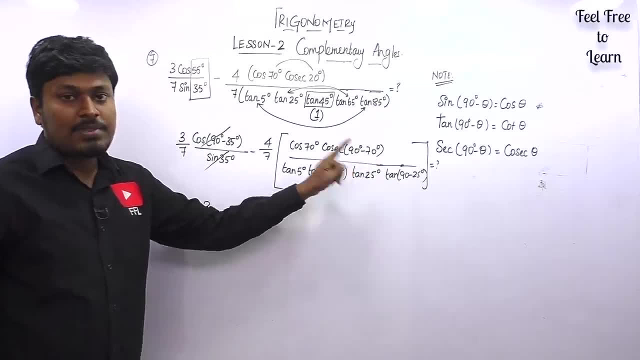 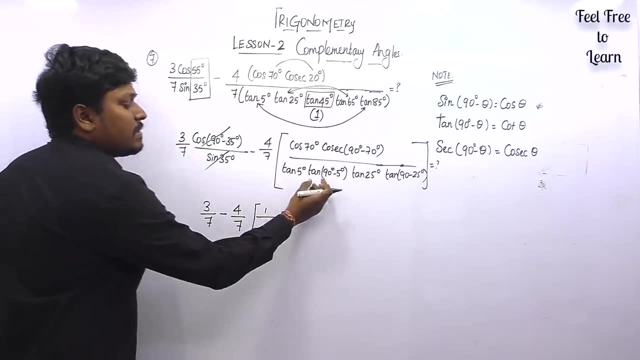 minus theta will be secant theta, secant 70 degree. So secant can be written as 1 by cos. So we can cancel cos and cos. here again the numerator is 1, divided by So. similarly, tan 90 minus theta will be cot theta, which is cot 5 degree. 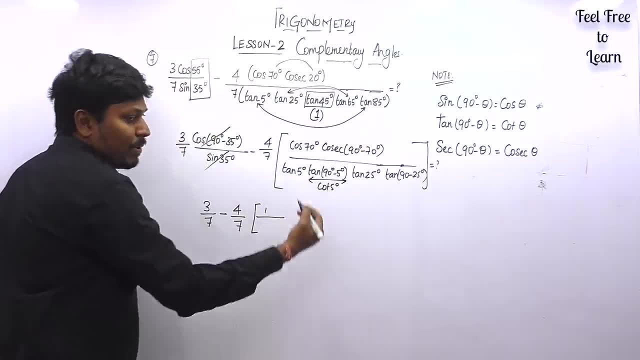 So this answer will be cot 5,. got it. So cot can be written as 1 by tan 5.. So tan 5, tan 5.. Again, we can cancel it. Again, we can cancel 25 and 25.. So finally we got a denominator as 1..